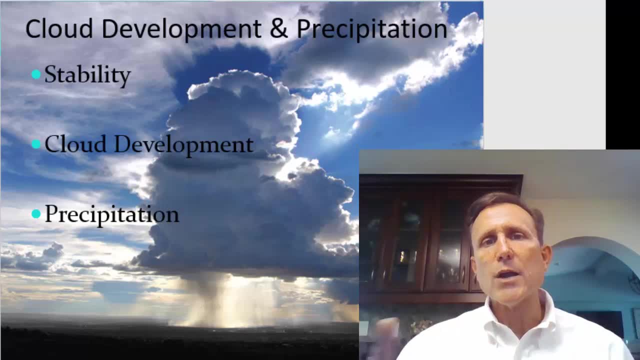 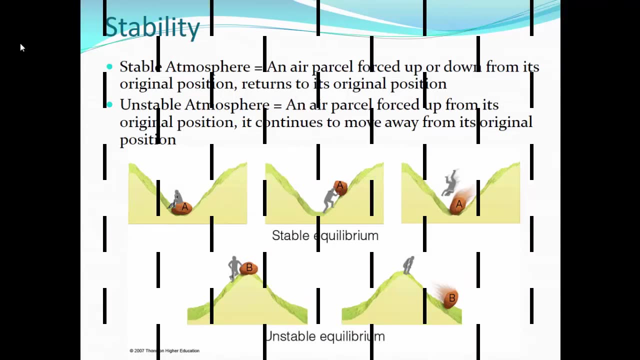 whether the parcel is stable or unstable, but it's about the entire atmosphere, whether it's stable or unstable. So let's talk a little bit about stability. Understand that stability: we're referring to the atmosphere, the air, the environment, not the parcel itself. When the atmosphere is stable, a parcel that is pushed up will return. 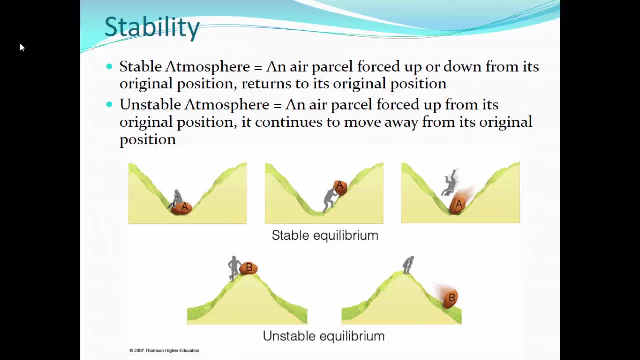 to its original position. And when the atmosphere is unstable, a parcel that is pushed will move away from its original position And you can see on the illustration the little man sitting on the big rock A in a stable equilibrium. When he pushes it up the hill it rolls back down the 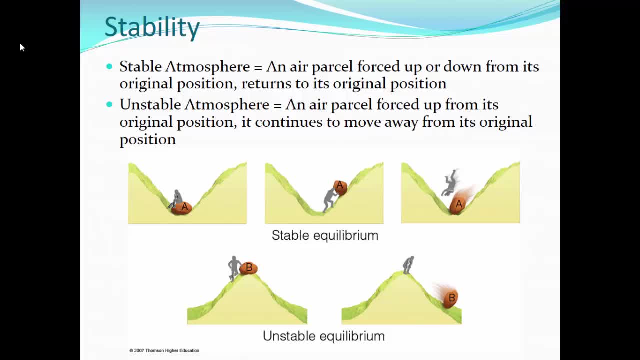 hill. But the little man at the top of the hill is in an unstable position And when he pushes it up the hill it's in an unstable equilibrium. So when he gives that rock a push it continues to roll down the hill- Stable air. when forced up or down from its original position, it returns to its 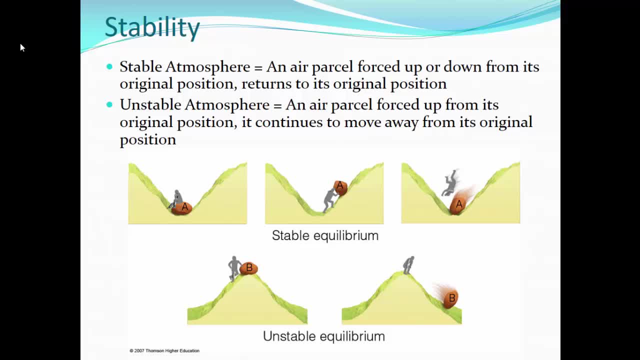 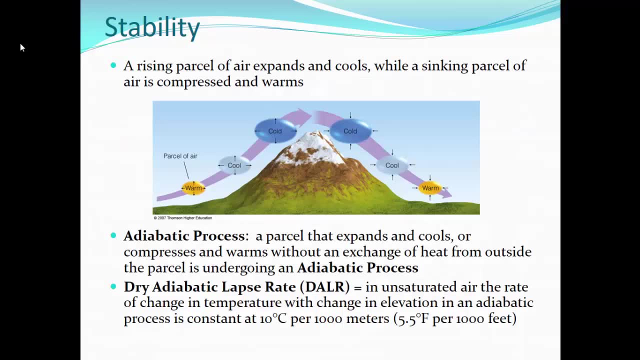 original position. And unstable air: when forced up or down from its original position, it continues to move away from its original position. So how does that play out with the weather and in the atmosphere? Well, as we know, a rising parcel of air expands and cools, while a sinking parcel of 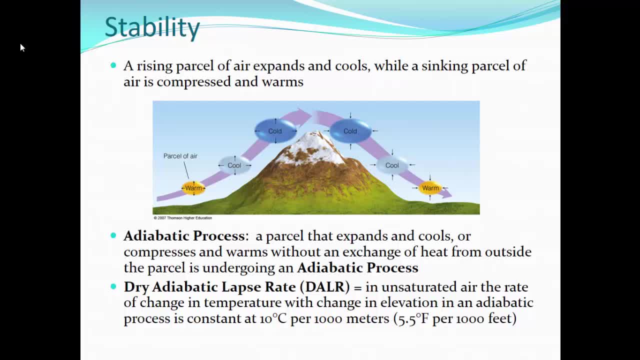 air is compressed and warmed And we can see our parcel going up the side of the mountain, being pushed up the side of the mountain from left to right. As it goes up in the atmosphere, the pressure lowers. As the pressure lowers, there's not as much pushing in in the parcel, so it expands And as 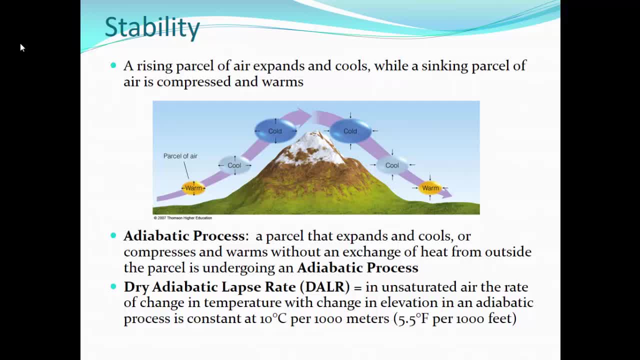 you learned from previous chapters, some of the energy used in pushing out that parcel is required and it cools the parcel And as the pressure goes down and the parcel expands bigger, it continues to cool. It of course happens when the parcel is forced down the mountain As pressure increases going down. 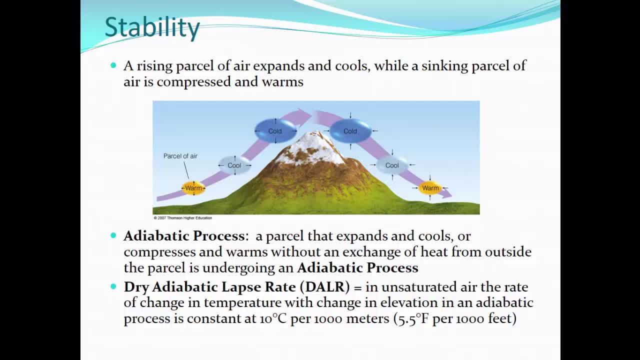 in elevation, the parcel is compressed, and that compression causes the molecules inside the parcel to begin to move more quickly. This process of warming or cooling without an actual exchange of heat is known as an adiabatic process. In an adiabatic process, a parcel that expands and cools or compresses 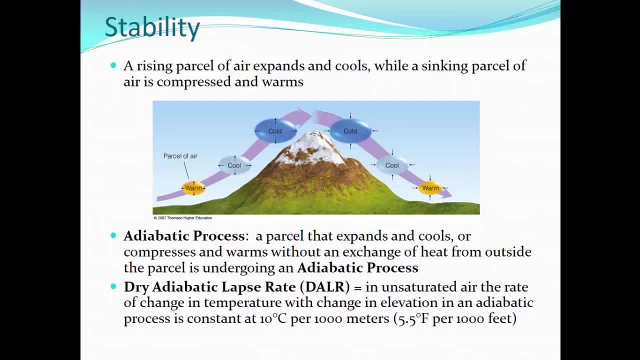 and warms the particles Without an exchange of heat from the outside of the parcel is undergoing that adiabatic process And in the atmosphere that change in temperature with height is a lapse rate And when the parcel is unsaturated or the relative humidity is less than 100%. 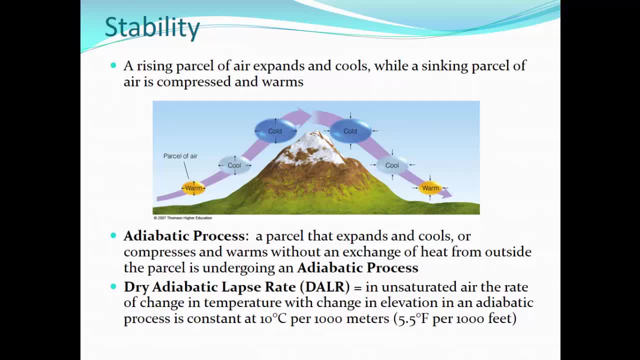 you have an unsaturated air parcel, The change in temperature with height is fixed And that is known as the dry adiabatic lapsed-rate. in unsaturated air the rate of change in temperature with the change in elevation in an adiabatic process is constant: 10 degrees Celsius per 1,000 meters. 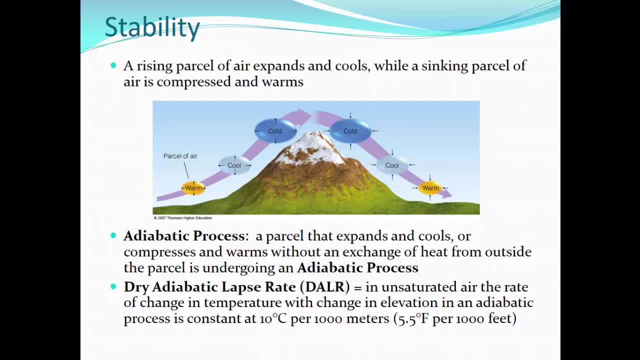 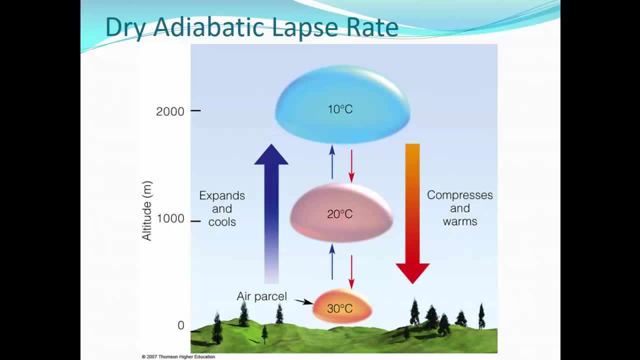 Also 5.5 degrees Fahrenheit per 1,000 feet, but 10 degrees Celsius per 1,000 meters. that's going to be easier math, Alright. so here is the dry adiabatic lapse rate in motion. Here's it happening. 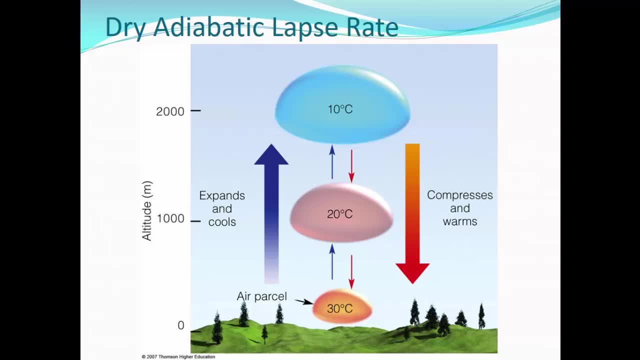 You start the parcel at the surface at 30 degrees Celsius. You force that parcel to rise 1,000 meters. It expands and cools and in that 1,000 meters it cools exactly 10 degrees Celsius. You force it up another 1,000 meters and it cools another 10 degrees Celsius, from 20 to 10 degrees. 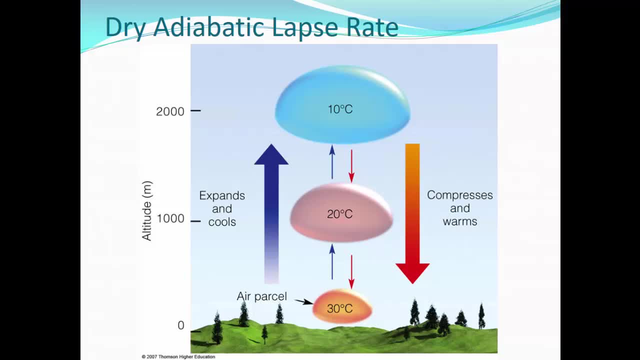 Same thing happens when you push that parcel back down. As you force it down from 2,000 feet to 1,000 feet, compression warms it by 10 degrees. As you force it down from 1,000 feet to the surface, compression warms it to 30 degrees Celsius. 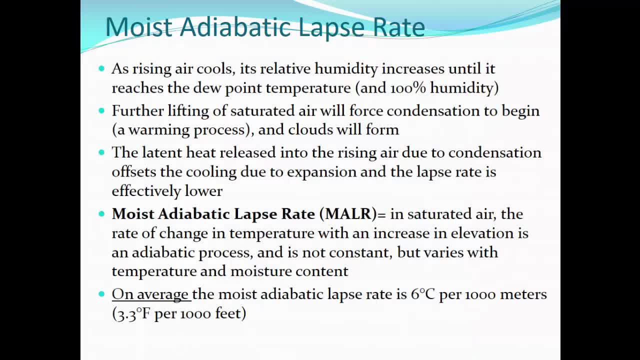 Alright. so if there is a dry adiabatic lapse rate for unsaturated parcels, parcels that have relative humidity less than 100%, then we also have to have a lapse rate for parcels that are saturated at 100% relative humidity, and that would be the moist adiabatic lapse rate. 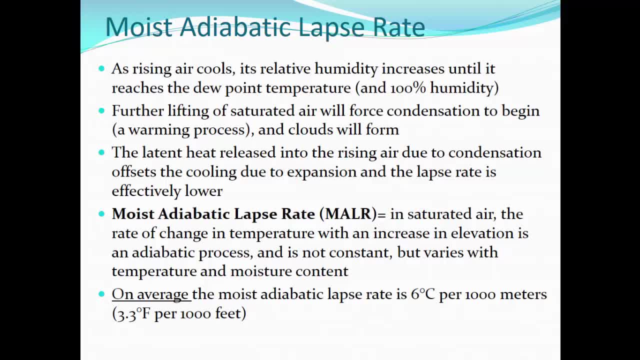 The moist adiabatic lapse rate is a little bit lower than the dry adiabatic lapse rate because in moist air, in saturated water, and the dry adiabatic lapse rate it's a little bit lower than the dry adiabatic lapse rate. 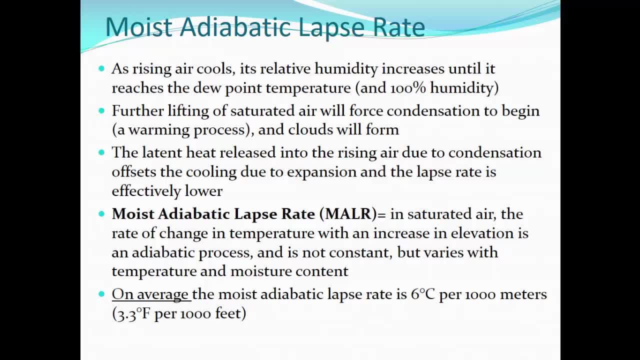 air, an air that has 100% relative humidity. if you force that air to rise, it will continue to cool and that will force condensation. And if you remember from Chapter 2, condensation is a warming process. So as rising air cools, its relative humidity increases until it reaches the dew point temperature in 100% relative humidity. 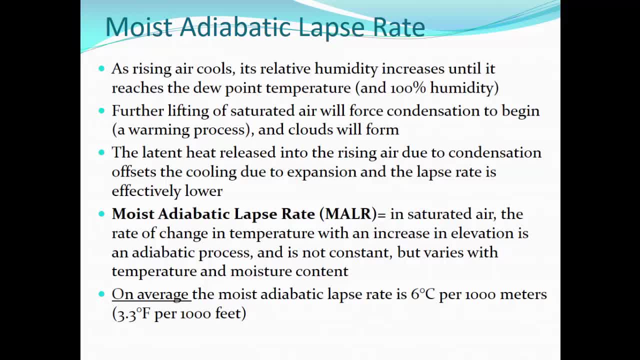 So again, you start with the parcel at the surface. its relative humidity is less than 100%. you force it to rise. it cools at 10 degrees Celsius per 1,000 meters until it gets to its dew point. And when it reaches its dew point it reaches 100% relative humidity. it is saturated. 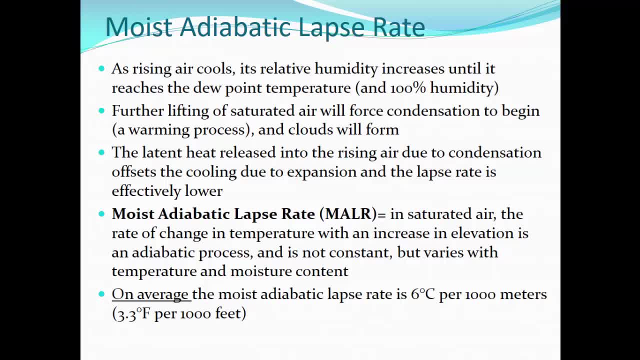 Further lifting of the saturated air parcel will force condensation to begin, which is a warming process, and clouds will form. The latent heat released into the rising air due to condensation offsets the cooling due to expansion and the lapse rate is effectively lower. 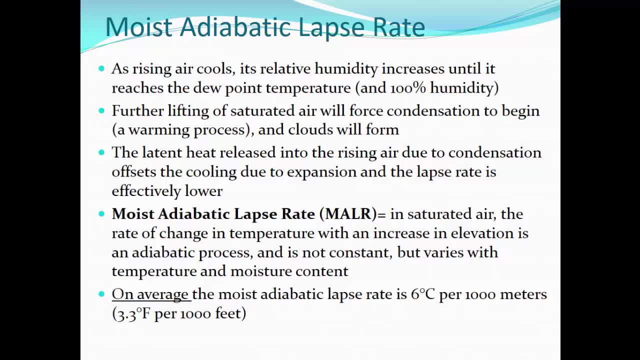 So in the moist adiabatic lapse rate in saturated air, the rate of change in temperature with an increase in elevation is an adiabatic process and is not constant but varies with temperature and moisture content. So on average the moist adiabatic lapse rate is about 6 degrees Celsius per 1,000 meters. 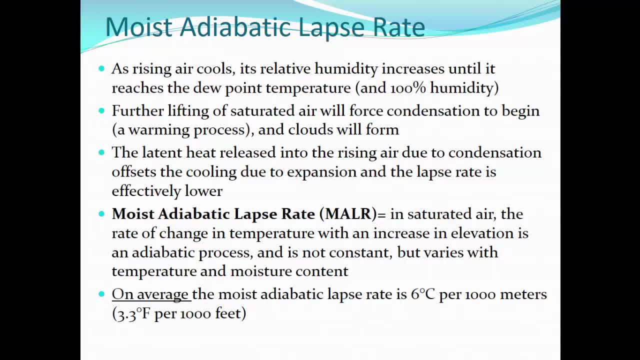 So it varies. it is not a constant. the dry adiabatic lapse rate was a constant at 10 degrees Celsius per 1,000 meters. the moist adiabatic lapse was constant: 10 degrees Celsius per 1,000 meters. 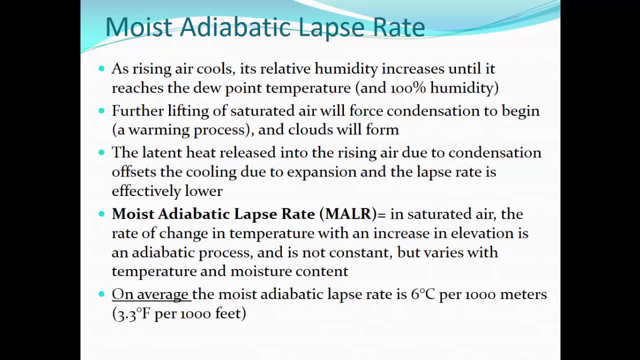 The adiabatic lapse rate is not. it varies. It varies with the amount of moisture and the temperature of the parcel to start with, Because the warmer the parcel is to start with, the more moisture that's available When condensation occurs, more heat can be released. So the moist adiabatic lapse rate effectively is variable. 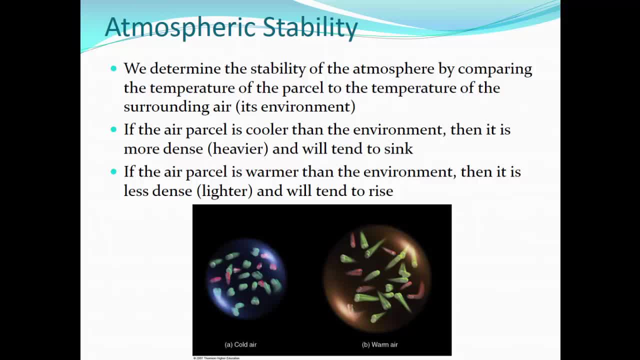 Atmospheric stability. we determine the stability of the atmosphere by comparing the temperature of the parcel to the temperature of the surrounding air, its environment. If the parcel is cooler than the environment, such as the parcel we see on the left, it's colder. the molecules are moving more slowly, it has less volume. 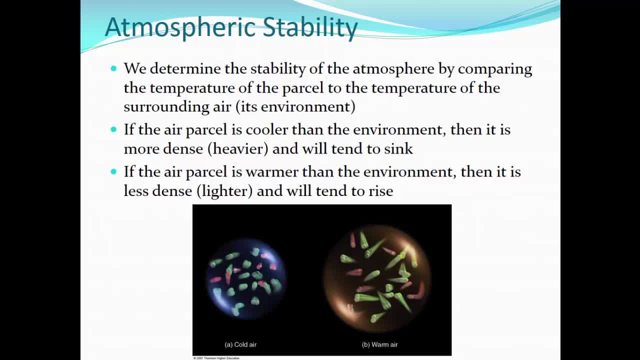 meaning it is more dense, then that parcel will tend to sink. It's more dense, it's heavier than air around it and it will tend to sink. Now, if that parcel is warmer than its environment, the molecules are moving more quickly. 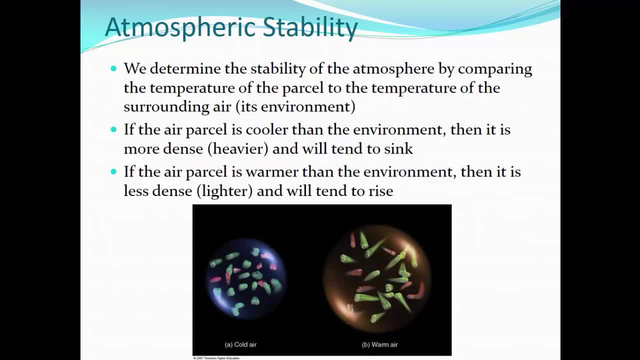 it's pushed out and it causes the parcel to expand. it's using more volume with the same amount of mass. its density is less. it's less dense, then it is lighter than the air surrounding it, the environment, and it will tend to rise. 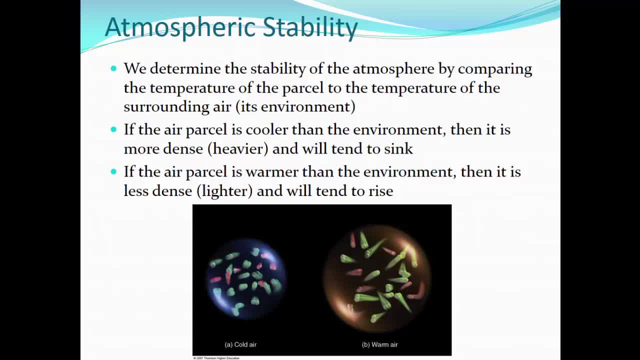 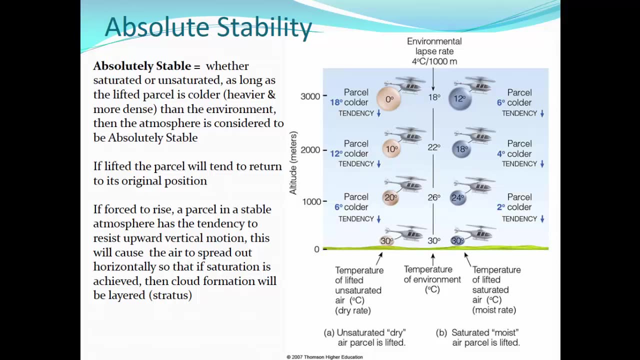 So the stability of the atmosphere is determined by comparing the temperature of the parcel to the temperature of the surrounding air. So let's start with an absolutely stable environment. This is to say that the entire atmosphere, the entire environment, is stable. Parcels that are forced up will tend to return to their original position. 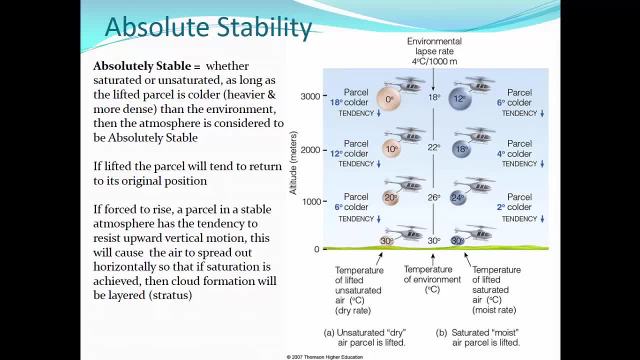 If they're pushed up, they will tend to sink back down. Why would they do that? Well, only if they're colder than their environment. If the environment and the environmental lapse rate is such that the lifted parcel remains colder than the environment, the parcel will tend to sink. 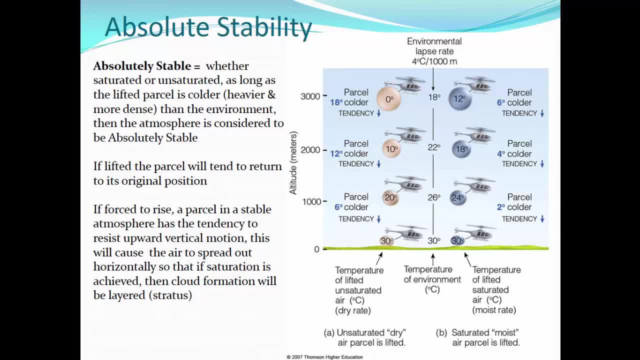 So look at our illustration. We have the environmental lapse rate right down the middle of 4.5 degrees Fahrenheit. So we have the environmental lapse rate right down the middle of 4.5 degrees Fahrenheit. So we have the environmental lapse rate right down the middle of 4.5 degrees Fahrenheit. 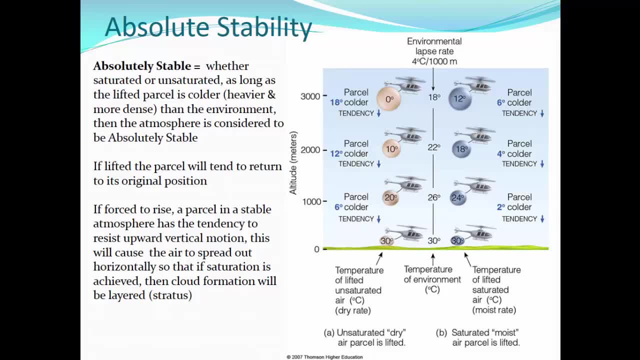 And the temperature we had already recorded is 4 degrees Celsius per 1,000 meters. Of course, that environmental lapse rate, that's a given. It's stated, It's what it is. It can be different in any location, any place, any time on Earth. 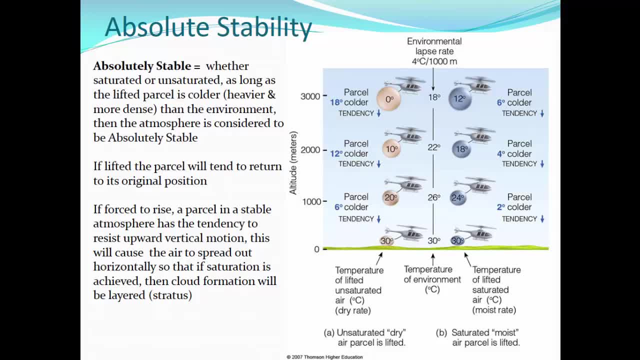 The degree to which the temperature decreases at the height is a variable thing based on atmospheric conditions. In this case it's 4 degrees Celsius per 1,000 meters, So it doesn't cool with height very quickly. On the left side we have the dry parcel. 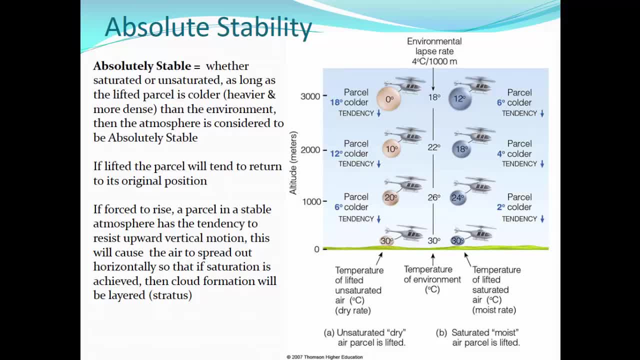 It is less than 100% relative humidity, so it cools at a dry adiabatic lapse rate. On the right side, The blue one, that's the moist parcel- It's 100% relative humidity, it's saturated, so it cools at 6 degrees Celsius per 1,000 meters. 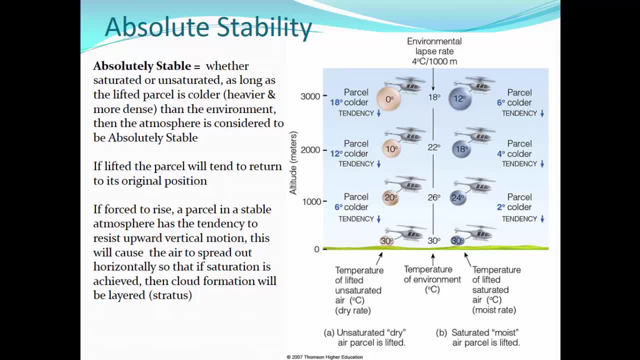 And you can see, as the parcel is lifted, by what, What's physically lifting that parcel? Well, the helicopter is. As the parcel is lifted, the dry parcel cools by 10 degrees Celsius per 1,000 meters to 20 degrees at 1,000 meters, 10 degrees at 2,000 meters and 0 degrees at 3,000 meters. 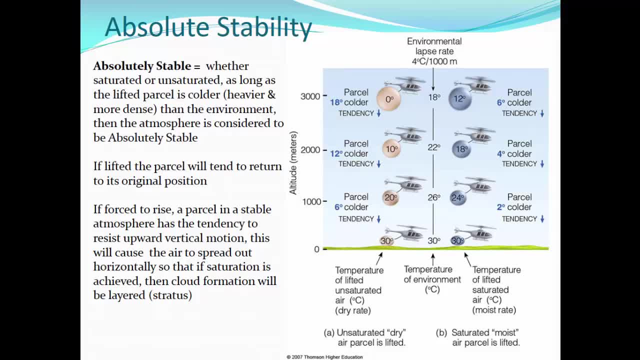 The moist parcel cools at 6 degrees Celsius per 1,000 meters, from 30 degrees to 24 degrees at 1,000 meters, 24 to 18 degrees at 2,000 meters and 18 to 12 degrees at 3,000 meters. 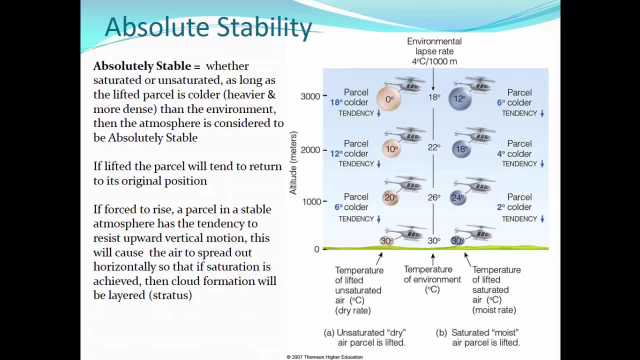 In each of those levels, the parcel, whether dry or saturated, remains colder than the environment and therefore will tend to sink. If lifted, the parcel will tend to return to its original position. Now with the saturated parcel, and even with the unsaturated parcel. 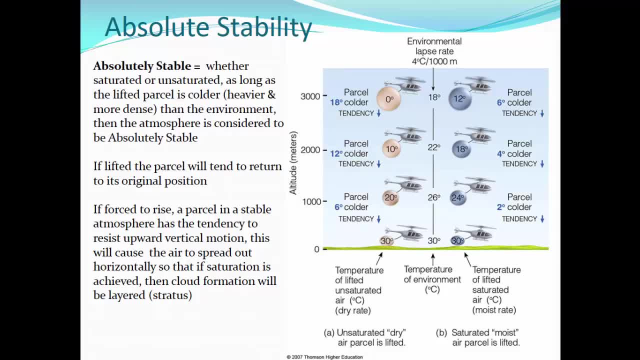 if the saturated parcel is forced to rise, condensation will occur. That's why the lobster rate is lower. What will happen with those clouds And in the dry parcel if it's lifted far enough that its temperature drops to its dew point? 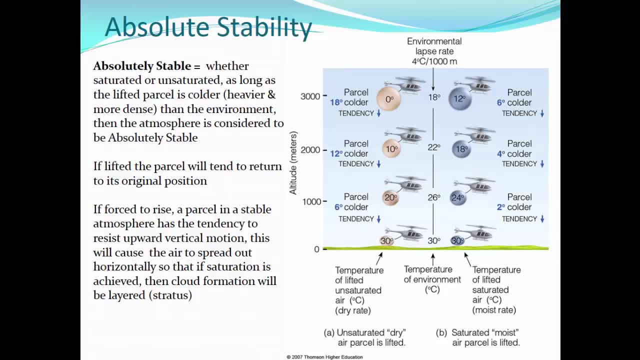 and condensation occurs because of it reaching 100% relative humidity, and cloud formation occurs. what will happen to those clouds If forced to rise? a parcel in a stable atmosphere has the tendency to resist upward vertical motion. This will cause the air to spread out horizontally. 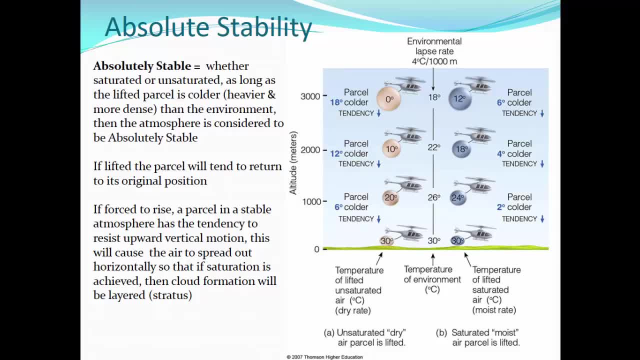 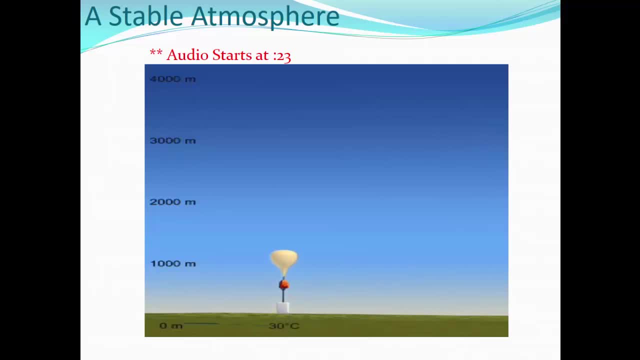 so that if saturation is achieved, then cloud formation will be layered or stratus clouds. The beginning of this particular animation is going to show you a radio sound, which is an instrument that measures temperature and humidity and wind speeds and radios it back to an observation station. 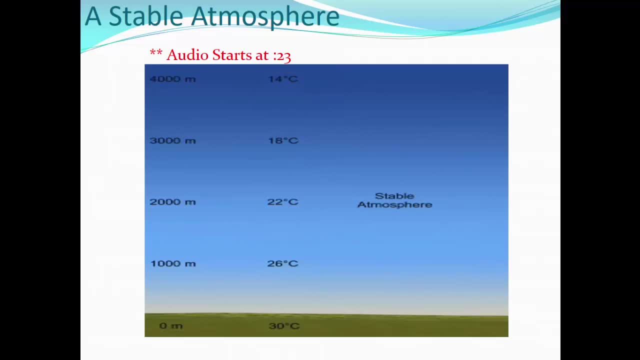 And it's being lifted by a weather balloon to get an idea of what the environmental lapse rate is, to show that it's a stable atmosphere. A stable atmosphere exists when the decrease in air temperature with height is less than the moist adiabatic rate. 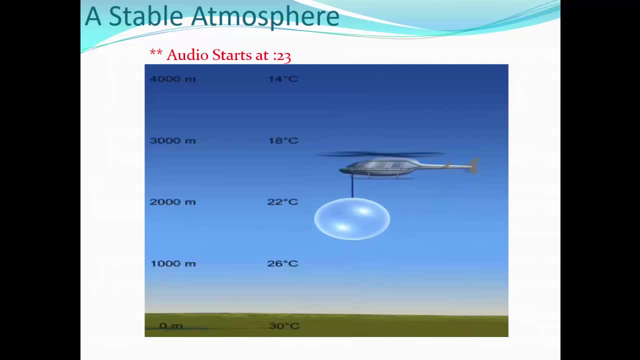 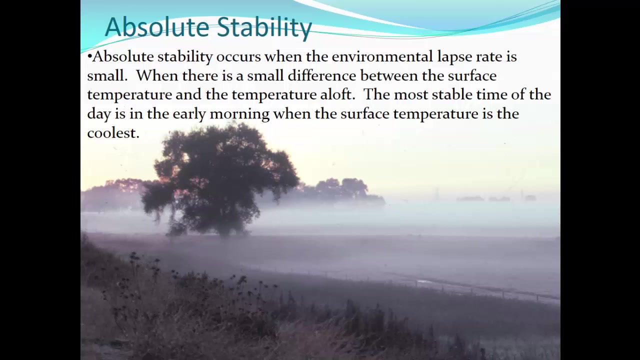 When this atmospheric condition occurs, the unsaturated air inside a lifted parcel will be colder, heavier and more dense than the air surrounding it. So when the parcel is released, it will fall back to its original position. So when the atmosphere is absolutely stable. 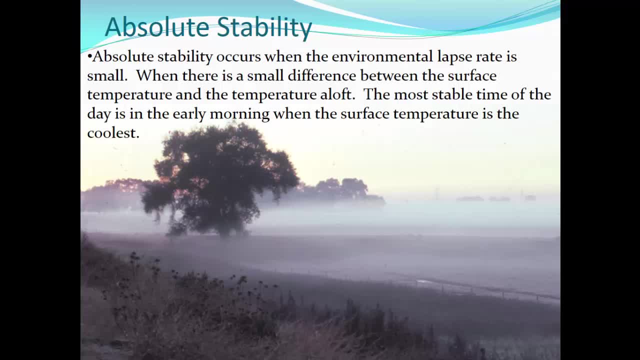 the environmental lapse rate is very small. There's very little cooling that goes on from the bottom of the atmosphere to the top of the atmosphere, And when would that typically be? Well, in the early mornings It's coolest just before sunrise. That's when the surface is as cool as it's going to get. 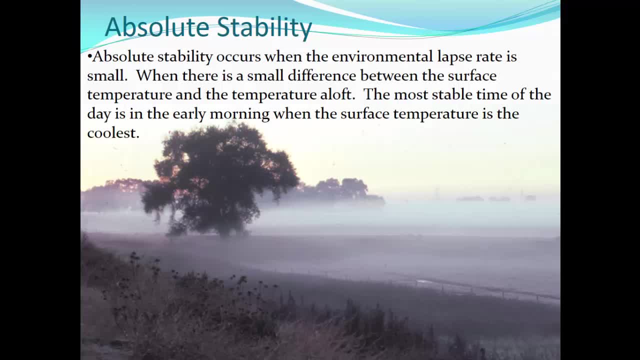 And aloft the temperature is pretty stable so they're cool as well. So there's a small difference between the surface cool temperature and the upper level cool temperature. So the parcel that's forced to rise will continue to be colder. It's going to rise at the dry adiabatic lapse rate or the moist adiabatic lapse rate. 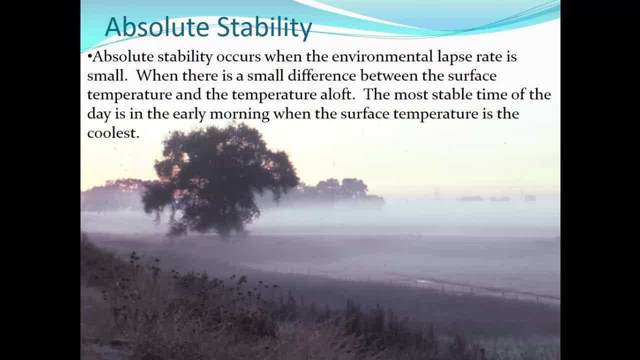 And it's going to tend to be colder than its environment and want to sink. And when those parcels reach saturation and cloud formation occurs. what you're left with are these type of clouds. This is kind of a mixture of fog and stratus clouds. 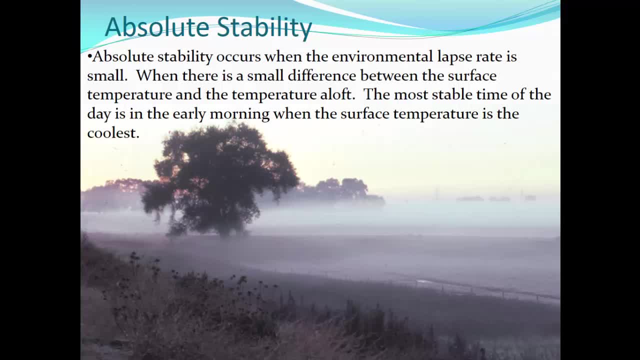 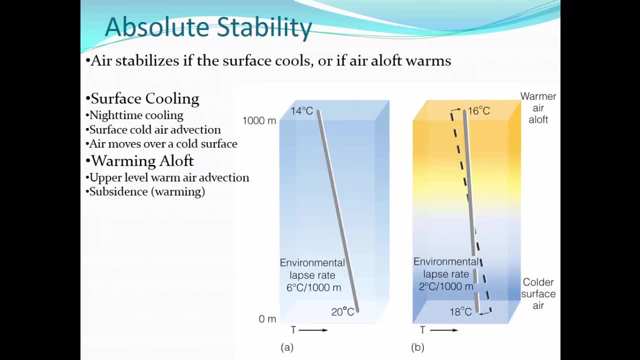 So the most stable time of day is early in the morning, when surface temperature is coolest, And that's when you get these nice low stratus clouds. So absolute stability. How do you stabilize the atmosphere? Look at the illustration on the right. The first box is the environmental lapse rate of 6 degrees Celsius per thousand meters. 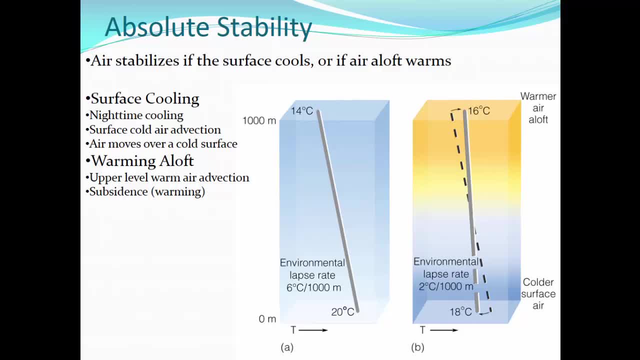 And then in the second box, we have cooled the surface by 2 degrees and warmed the air aloft by 2 degrees, And so our 6 degree Celsius per thousand meter environmental lapse rate has decreased to 2 degrees Celsius per thousand meters. 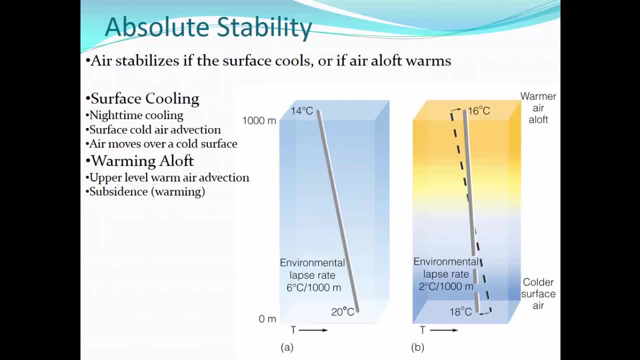 And by cooling the surface or warming the air aloft, you stabilize the atmosphere Again. the parcel at the surface is going to cool, if it's dry, at 10 degrees Celsius and always be colder than the environment. And even if it's moist, it's going to cool at 8 degrees Celsius and still always be colder than the environment. 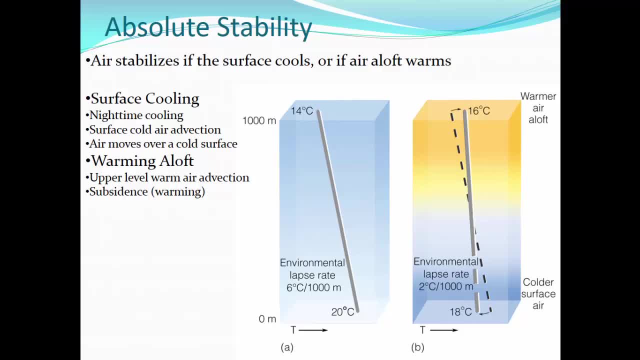 So you can stabilize the atmosphere by cooling the surface or warming it up aloft. Now how do you do those two things? Well, of course, at nighttime you cool the surface. You can also cool the surface with cold air advection. 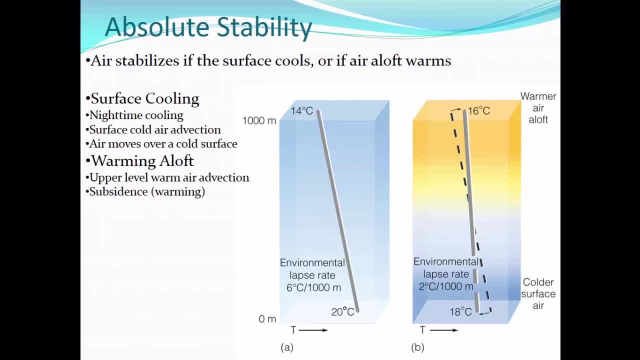 A cold front moves by and north winds blow in colder air And you can also cool the surface. if warm air moves over a colder surface, It will tend to chill that air at the bottom. That will stabilize the atmosphere. Now you can also warm things up aloft. 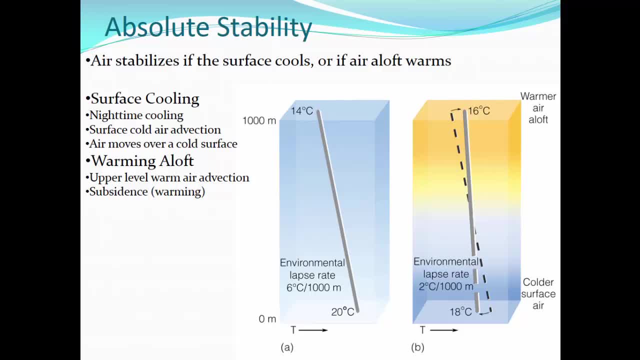 And the primary way to warm things up aloft is known as subsidence or warming. High pressure aloft is generally associated with warmer air aloft And high pressure aloft or warmer air aloft will create that stability and upper level warm air advection. 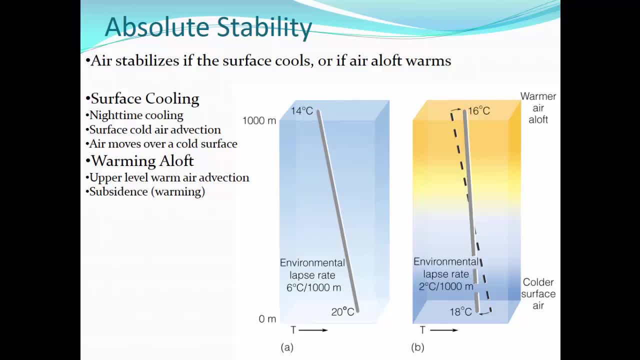 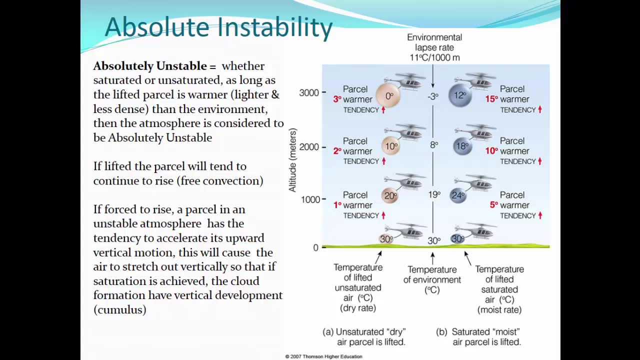 Warm air can actually be moved in in the upper levels, And that will also create stability, Absolute instability in unstable atmosphere. Look at our illustration. The environmental lapse rate is now significantly larger- 11 degrees Celsius per 1000 meters When parcels are lifted, because the atmosphere cools more quickly. 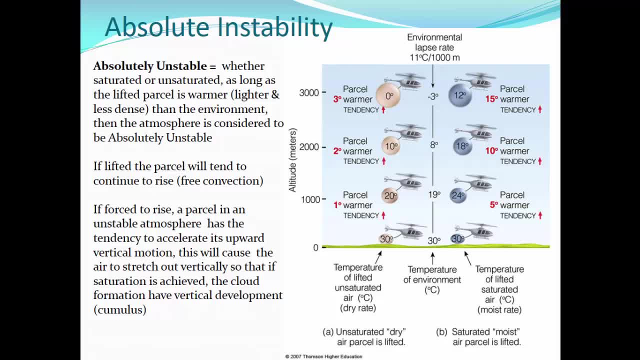 those parcels will be warmer at each level And therefore will want to continue to rise. So, just like with the stability illustration, we used a helicopter to get things moving, But truly, in this situation, because the parcel continues to be warmer than the atmosphere at each level. 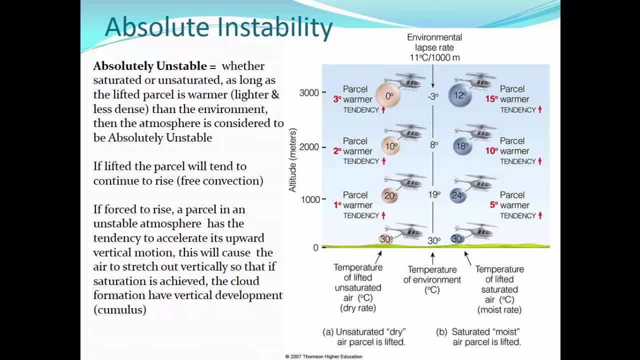 the parcel will rise on its own. So we take the dry parcel on the left, the saturated parcel on the right, cool the dry one at the dry adiabatic lapse rate to 1000 meters, 2000 meters to 3000 meters. 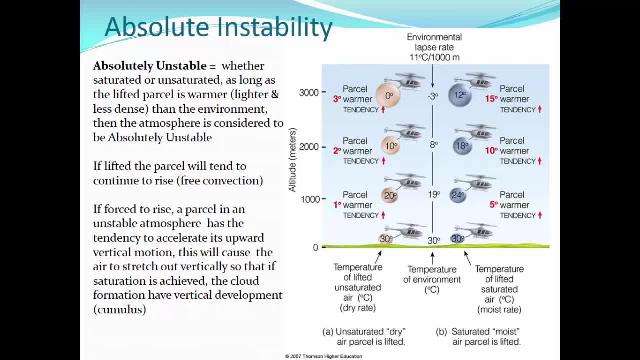 The same 20,, 10,, 0 degree, 0 degree range. And then also with the saturated Same thing happens. The saturated cools by 6 to 24 to 18 to 12. But at each level because of that much larger environmental lapse rate. 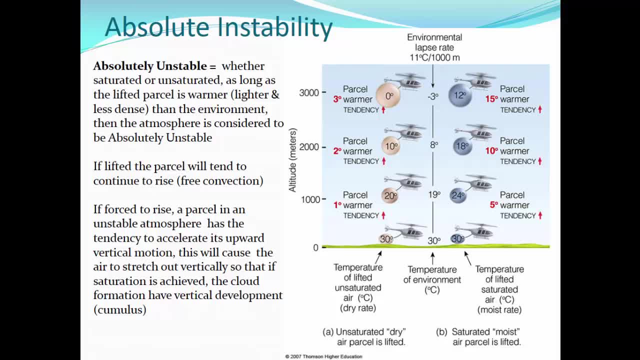 those parcels are warmer than the environment and will want to tend to rise, Whether saturated or unsaturated. as long as the lifted parcel is warmer, lighter and less dense than the environment, then the atmosphere is considered to be absolutely unstable If lifted. 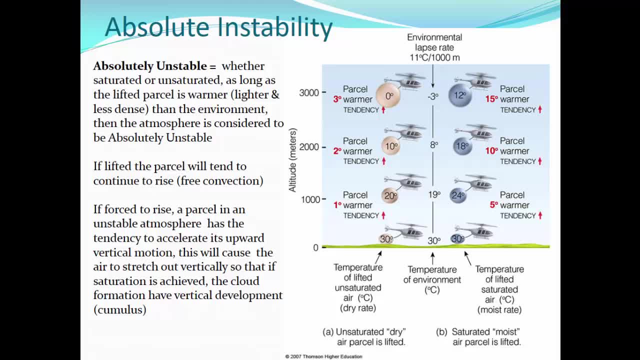 the parcel will tend to continue to rise- That is known as free convection- If it gets started being lifted and will continue to rise all on its own. we call that free convection If forced to rise the parcel in an unstable environment. 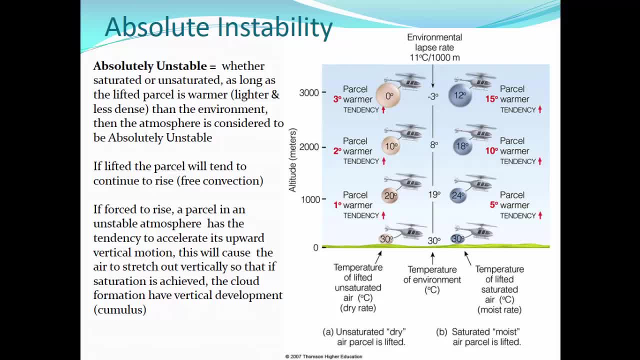 has the tendency to accelerate its upward vertical motion. This will cause air to stretch out vertically so that, if saturation is achieved, cloud formation will have vertical development and be cumulus clouds. The beginning of this illustration, this animation, is going to show the radio sun. 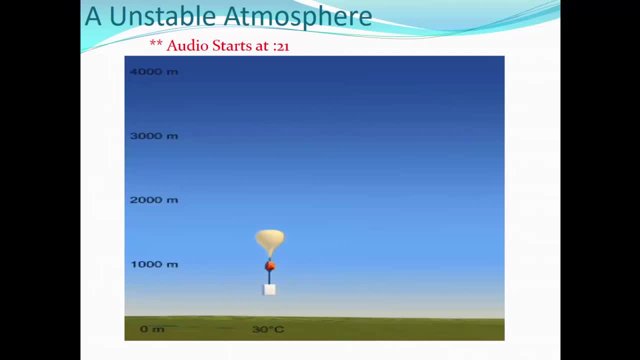 measuring the atmosphere using the weather balloon, And it's going to indicate an unstable atmosphere. This is an atmosphere where the parcel is going to want to continue to rise, And this is the type of atmosphere that we oftentimes have here in Central Florida, where air parcels rise all on their own. 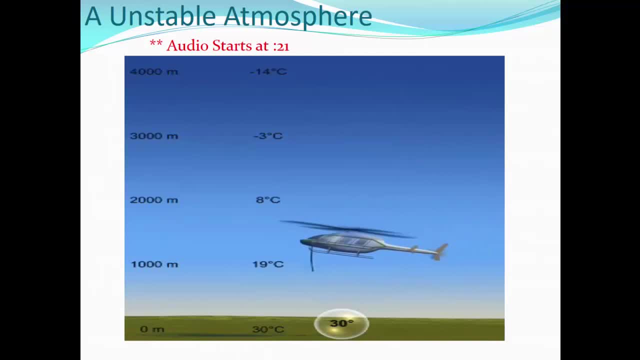 An unstable atmosphere exists when the decrease in air temperature with height is greater than the dry adiabatic rate. When this atmospheric condition occurs, the air inside the lifted parcel will be warmer, lighter and less dense than the air surrounding it. So when the parcel is released, 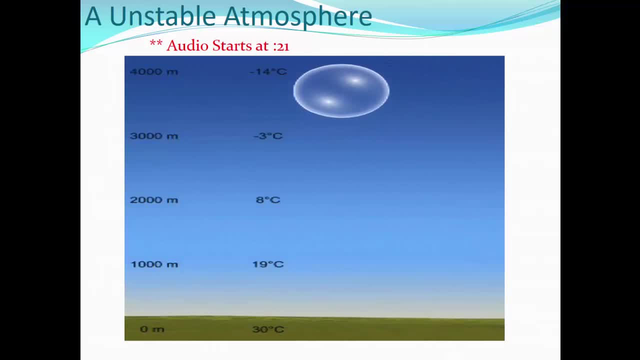 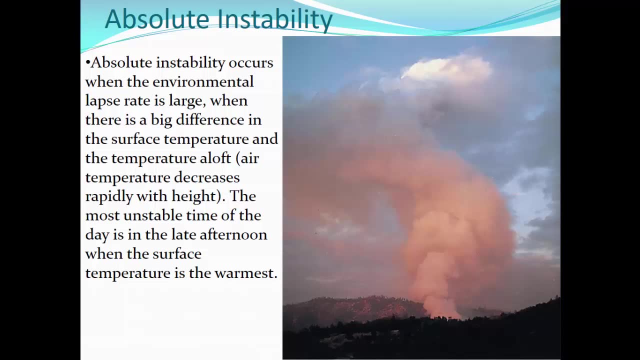 it will continue to rise away from its original position. Absolute instability occurs when the environmental lapse rate is very, very large, when there's a big difference in the surface temperature and the temperature aloft. Air temperature decreases very rapidly with height And that means that that parcel, if lifted, 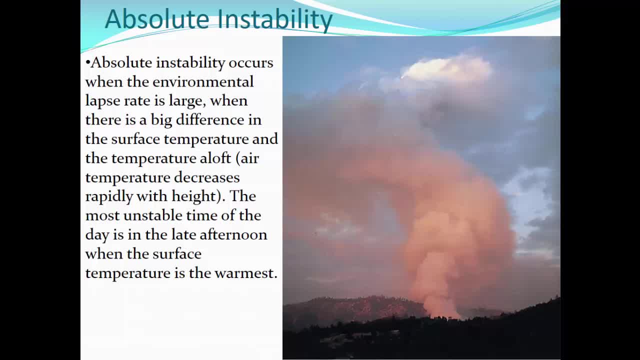 will continue to be warmer than the air around it, than the environment around it, and will want to continue to rise. The most unstable time of the day is in the late afternoon, when the surface temperature is in the warmest. Three, four o'clock in the afternoon. 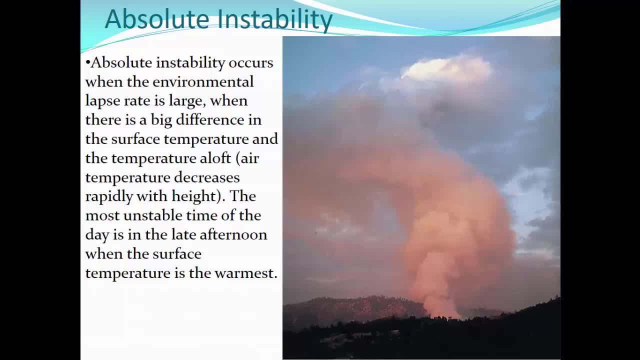 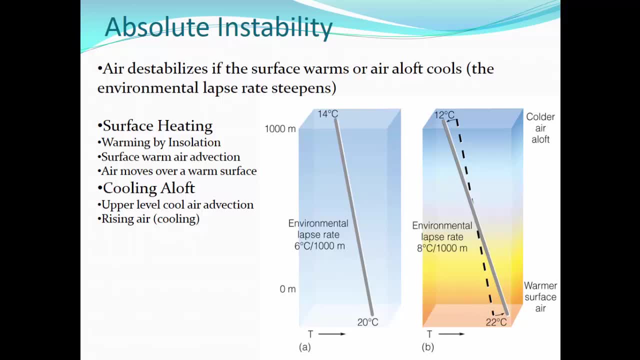 surface temperature is 80,, 85,, 90,, 95 degrees. That is when parcels will want to rise very quickly and they will tend to be warmer than the environment. So, in the same way that you can stabilize the environment by cooling it at the surface, 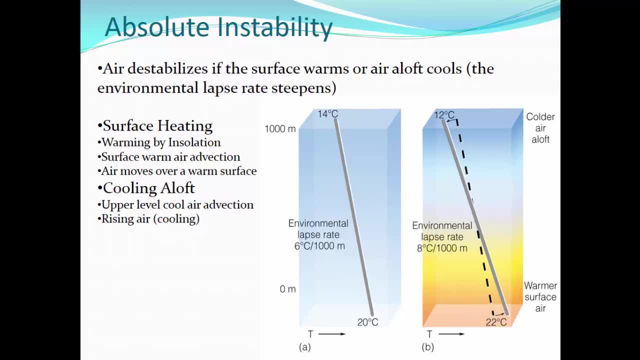 or warming it aloft. you can destabilize the environment by warming the surface, as in during the late afternoon, or cooling it aloft, And this concept of warm at the surface and cold aloft, creating an unstable atmosphere, is very important to our afternoon thunderstorms. 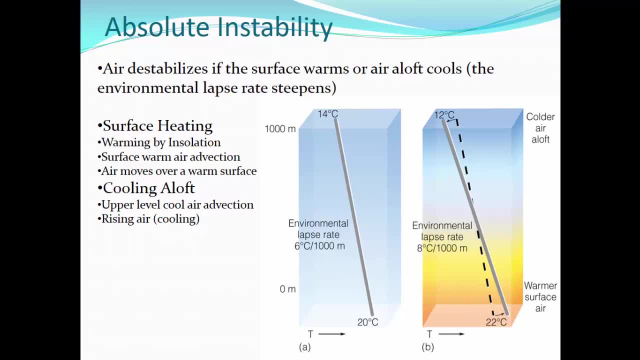 here in Central Florida, Air destabilizes. if the surface warms or if the air aloft cools, That means the environmental lapse rate steepens And in this situation we warm up the surface from 20 to 22, and we cool it aloft from 14 to 12,. 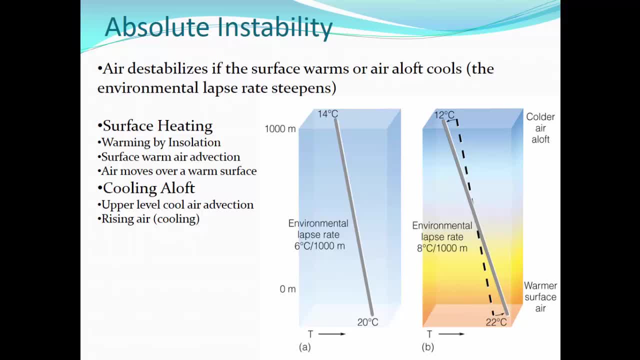 and our environmental lapse rate increases significantly, And that means that air that is forced to rise will tend to be warmer than the environment and continue to rise on its own. So how do you heat up the surface? Well, afternoon heating, warming by insulation. 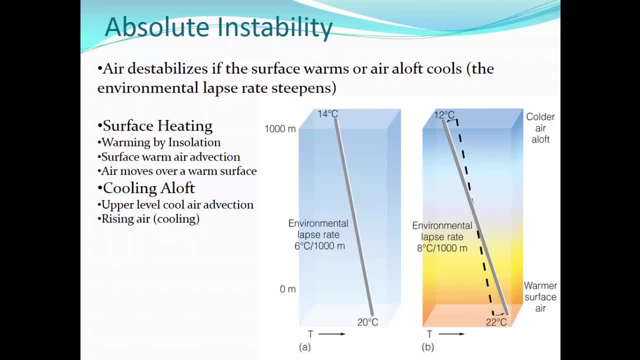 You can also have warm air advection, a nice deep south wind that can bring in warm air and destabilize the atmosphere, Or air can move over a warm surface and destabilize the atmosphere, such as colder air moving over a much warmer surface. 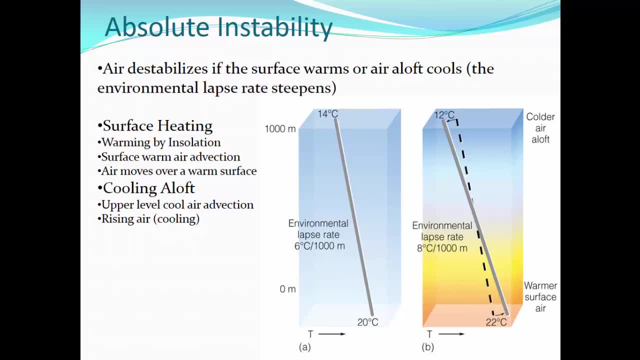 Now, how do you cool things up aloft? Well, upper level cool air, advection, air moving in horizontally in the upper levels of the atmosphere- that's a possibility- And rising air, or cooling due to rising air that is being forced to rise. 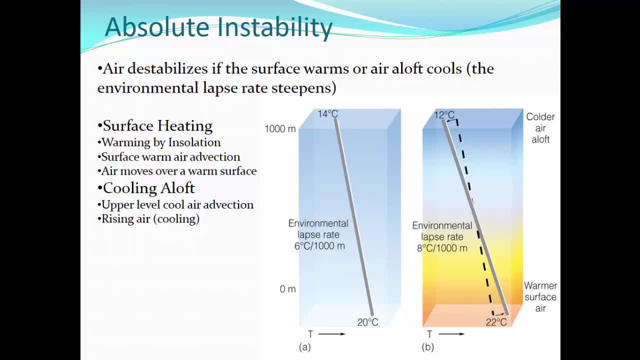 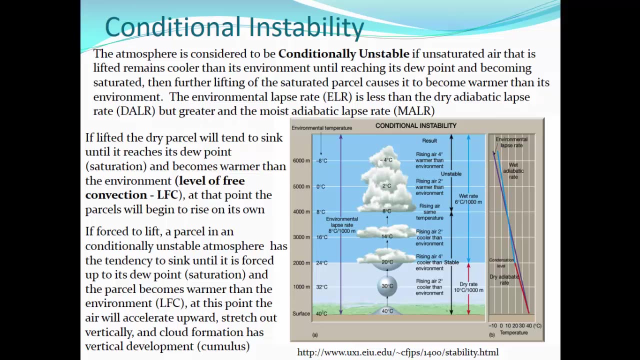 so a low pressure in the upper levels- Typically low pressure in the upper levels- is associated with cooler air aloft and that will destabilize the atmosphere. So an upper level low can destabilize the atmosphere and bring stormier conditions. Alright, so conditional instability. 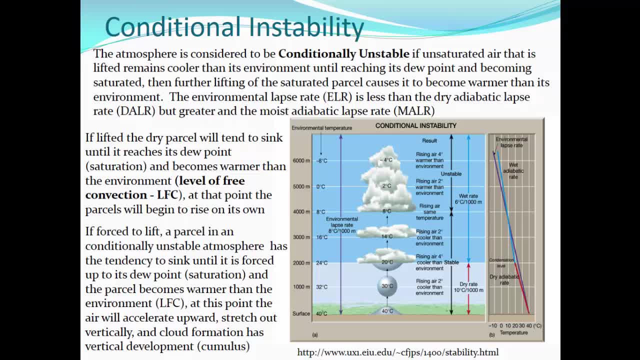 somewhere between an absolutely stable environment and an absolutely unstable environment, And this is where the atmosphere usually is. The atmosphere is considered to be conditionally unstable if an unsaturated parcel that is lifted remains cooler than its environment until it reaches its dew point and becomes saturated. 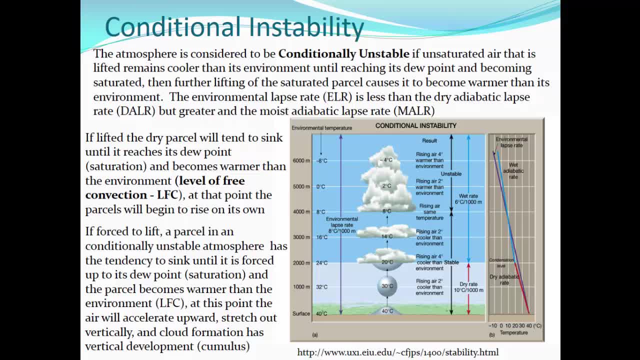 when further lifting of the saturated parcel causes it to become warmer than its environment. The environmental lapse rate is less than the dry adiabatic lapse rate, but greater than the moist adiabatic lapse rate. So what is that telling us? 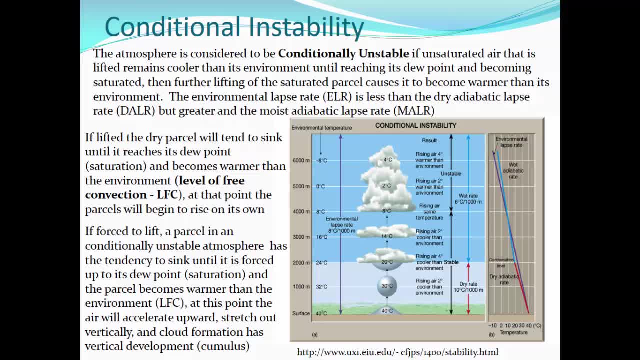 Well, look at this parcel. This is a little bit of a different illustration, but our environmental lapse rate over on the left this time is 8 degrees Celsius per 1,000 meters. So the dry parcel at 40 degrees Celsius at the surface. 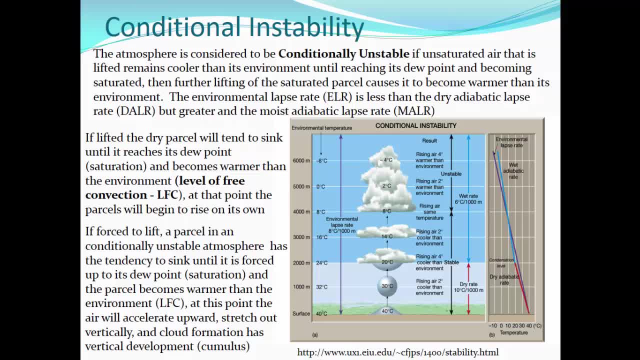 as it is forced to rise to 1,000 meters, it is still cooler than the environment, So it would want to sink. And even up to 2,000 meters, it is cooler than the environment and would want to sink, Something that is not defined on this illustration. 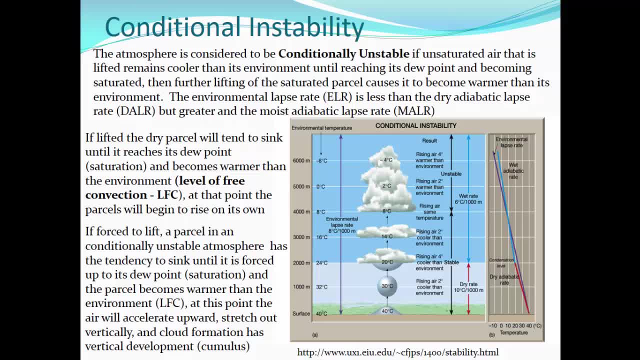 but we can tell by looking at it is. the dew point of this parcel is 20 degrees Celsius, And we know that because at 20 degrees Celsius condensation and cloud formation begins to occur. So at 20 degrees Celsius, or 2,000 meters. 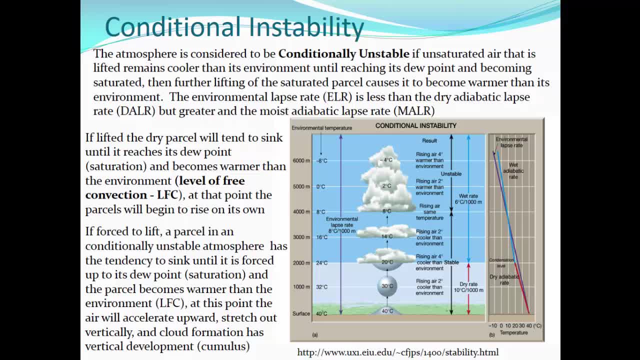 the parcel is no longer cooling at the dry adiabatic lapse rate. Now it's cooling at the moist adiabatic lapse rate. So you can see on the left-hand side that the red dry adiabatic lapse rate is the cooling rate up to 2,000 meters. 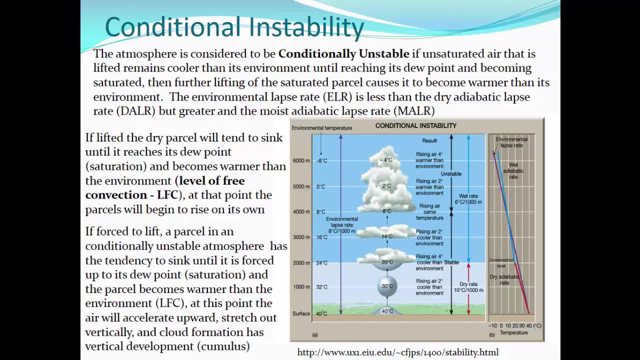 Then above it, it's cooling at the wet adiabatic lapse rate because that parcel has achieved saturation. So it's lifted now from 2,000 to 3,000 meters, but the parcel is still cooler than the environment. So we're still in a stable situation. 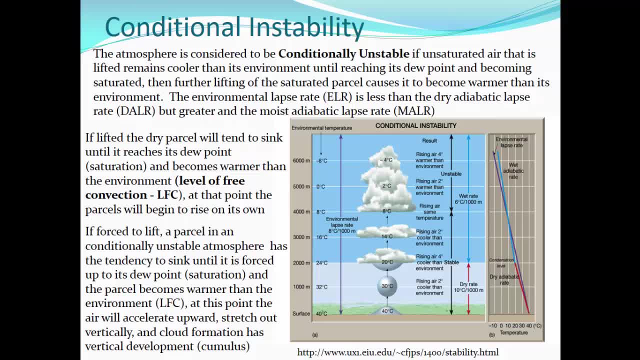 And even from 3,000 to 4,000 meters, the environment is cooler than or right at 4,000 meters, the same temperature as the environment, the parcel and the environment. So right on up to 4,000 meters. 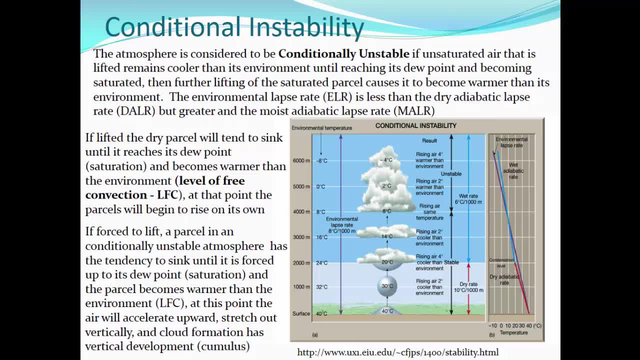 it is still a stable environment. But you'll notice that from 4,000 to 5,000, now- the environmental lapse rate is such that the saturated parcel cooling at the wet adiabatic lapse rate only cools at 2 degrees Celsius. 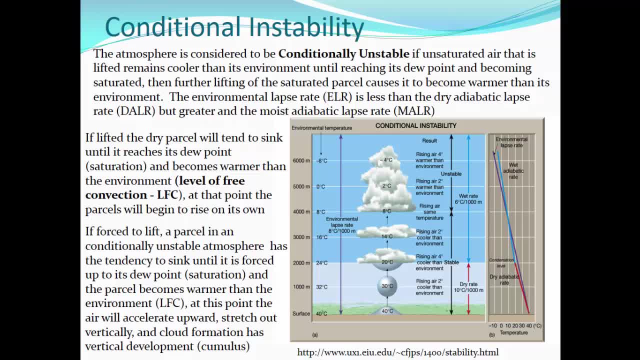 So between 4,000 meters and 5,000 meters the rising parcel is warmer than the air around it, and so it's an unstable environment. So it's stable from the surface to 4,000 meters and then unstable from the 4,000 meters all the way up. 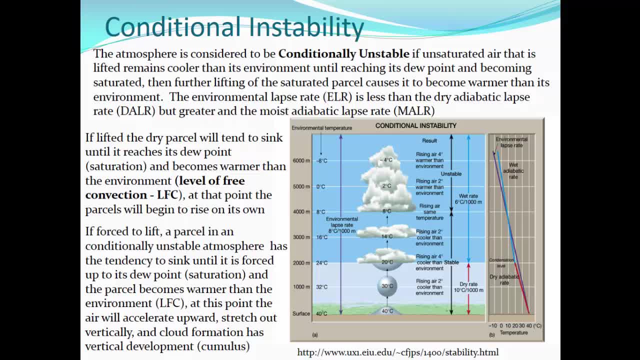 So the cloud formation at 2,000 meters and at 3,000 meters is stratus, flat layered clouds, because that air wants to resist upward motion. But once it gets to 4,000 meters the air begins to rise all on its own. 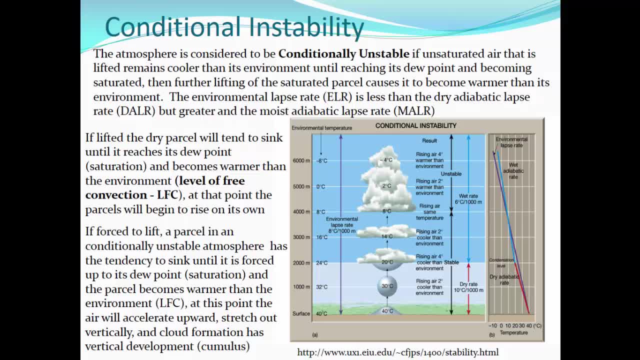 That's that free convection. And then with that, that upward motion of the air creates those clouds with vertical extent, or the cumulus clouds. So if lifted, the dry parcel will tend to sink until it reaches its dew point, saturation. 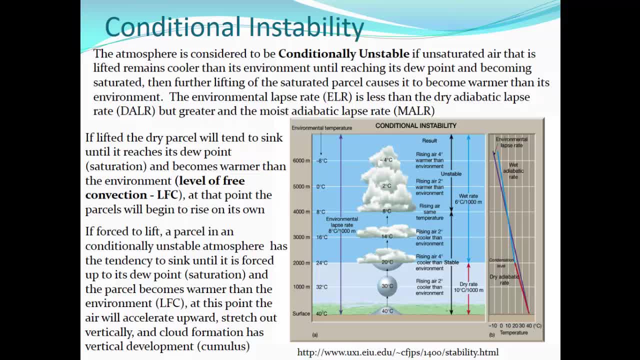 and becomes warmer than the environment. That is the level of free convection, And in the case of this illustration, that level of free convection is at 4,000 meters. At that point, the parcel begins to rise on its own. 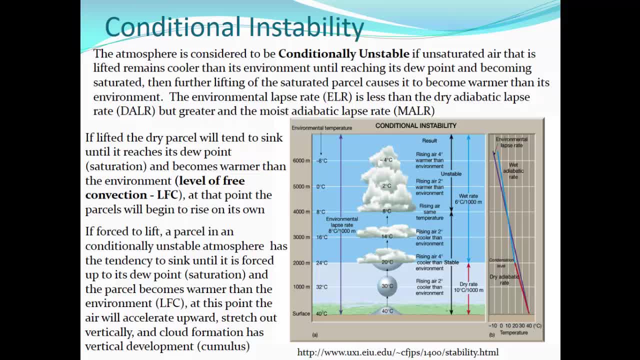 If forced to lift a parcel in a conditionally unstable atmosphere has the tendency to sink until it is forced up to its dew point- saturation- and the parcel becomes warmer than the environment at the level of free convection. At this point the air will accelerate upward. 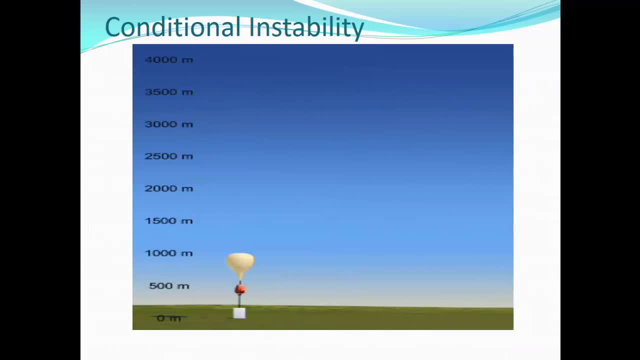 stretch out vertically and cloud formation has a vertical development and tends to be cumulus. A conditionally unstable atmosphere exists when the decrease in air temperature with height falls between the moist and the dry adiabatic rate. A conditionally unstable atmosphere may become unstable. 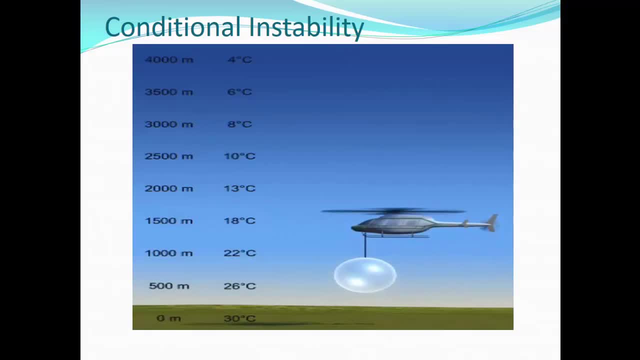 if a rising air parcel becomes saturated and a cloud forms, The latent heat released inside the cloud warms the air to the point that the rising air is now warmer and less dense than the air surrounding it. The cloud will continue to build until the rising air inside the cloud. 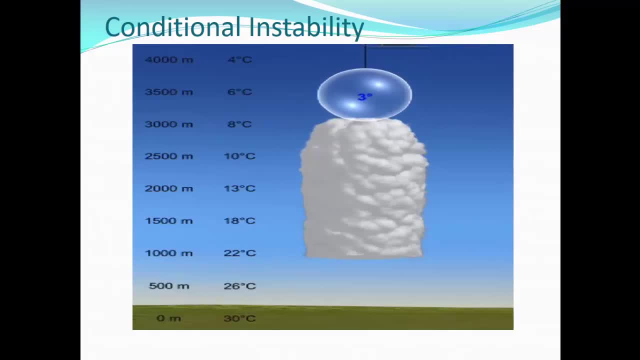 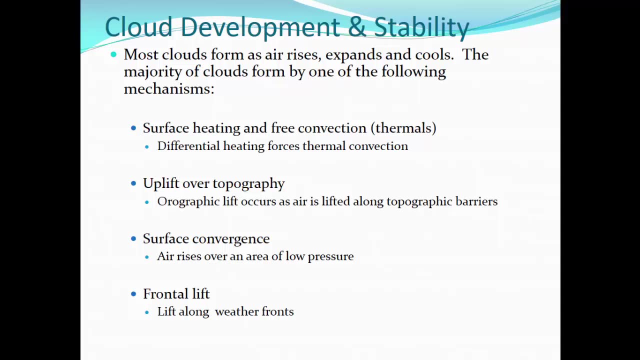 becomes the same temperature as the air surrounding the cloud. Alright, so we know that cloud formation occurs when an unsaturated parcel is forced to rise until it reaches its dew point. Once it reaches its dew point, it is at 100% relative humidity. 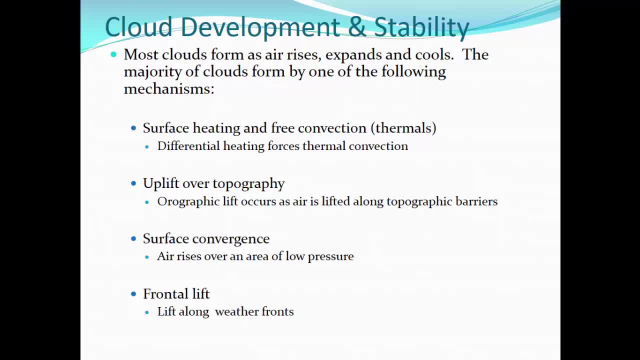 and further lifting will cause condensation and cloud formation. If that further lifting occurs in a stable environment, our clouds will be stratus clouds. If that lifting occurs in an unstable environment, then our clouds will be cumulus clouds. What causes that parcel to rise? 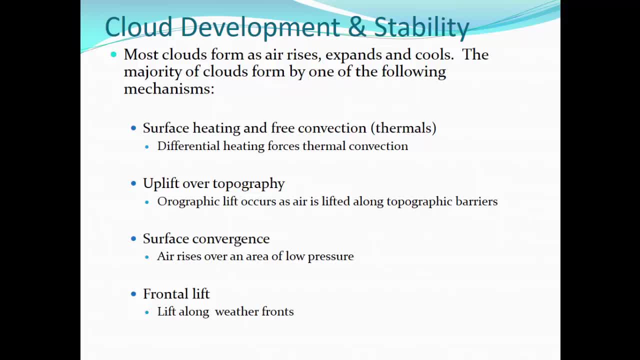 What causes the lifting? Well, in our illustrations we had helicopters. Helicopters don't cause air parcels to rise. How does it occur? in nature? Most clouds arise as air rises, expands and cools. The majority of clouds form by one of the following four mechanisms: 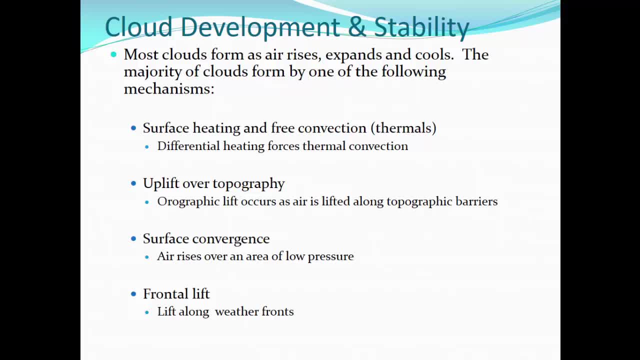 Surface heating, or what's known as free convection or thermal heating, means different heating at different points in the ground. one spot is hotter and the air over that spot tends to rise. You also have uplift over topography- All those pictures you've seen up to now. 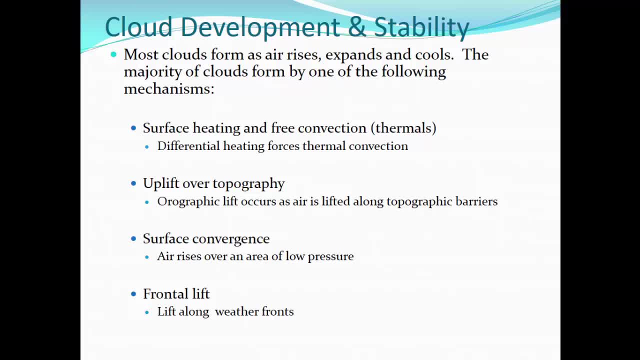 of wind going up and over mountains. that is, uplift over topography. This is known as orographic lift. It occurs as air is lifted along topographic barriers. The other way we can lift a parcel is through frontal pressure surface convergence- whether it is an actual low. 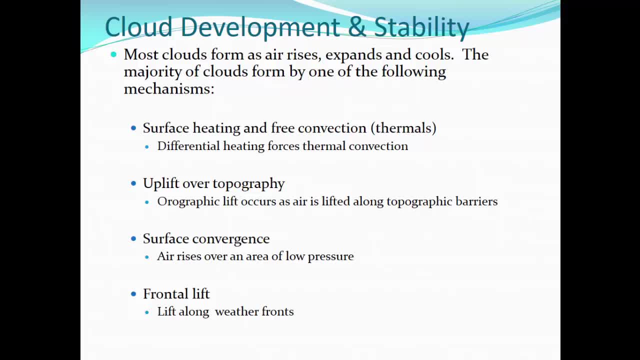 big red L on the weather map or it's a frontal boundary. Remember fronts are elongated areas of low pressure. So the fourth method of lifting is lifting along weather fronts. Four ways air is lifted: Surface heating, orographic lift. 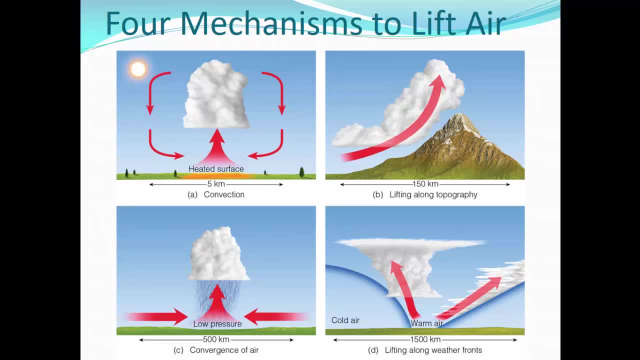 low pressure or frontal lift. So here are the four mechanisms to lift air On the upper left-hand side. that's your free convection. the heated surface, The dry parcel, rises less than 100% relative humidity. It rises right up to that cloud base. 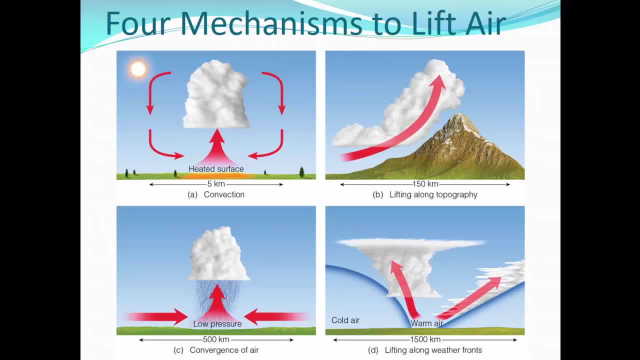 At that cloud base. the temperature is cooled by expansion to the dew point or 100% relative humidity, said to be saturated. Further lifting causes condensation and cloud formation. On the right there's your uplift over topography, your orographic lift. 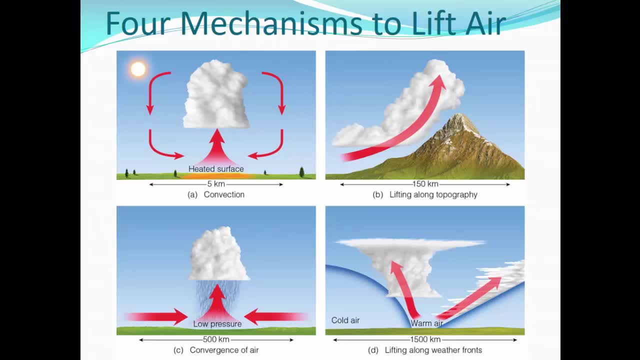 Converging air, low pressure at the surface surges on it and that creates your lift, Or the bottom right being lifted over a cold front to the left and a warm front to the right, And you can see that, those two different types of lift. 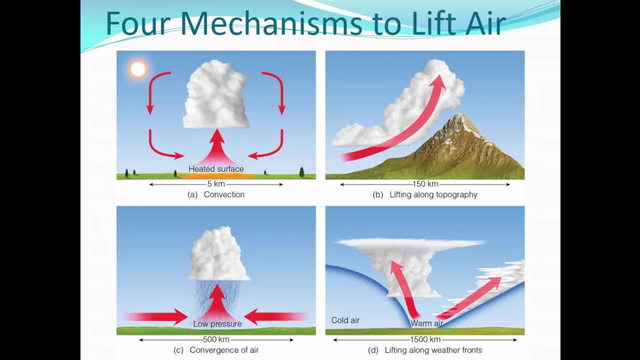 create two different types of clouds Because when the cold air moves over the warm surface, you have destabilized the atmosphere. Remember, a warm surface and cold air aloft destabilizes the atmosphere and there you get that cloud with vertical extent, Whereas with the warm front. 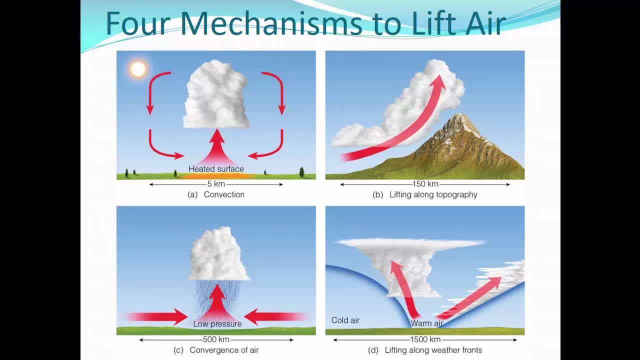 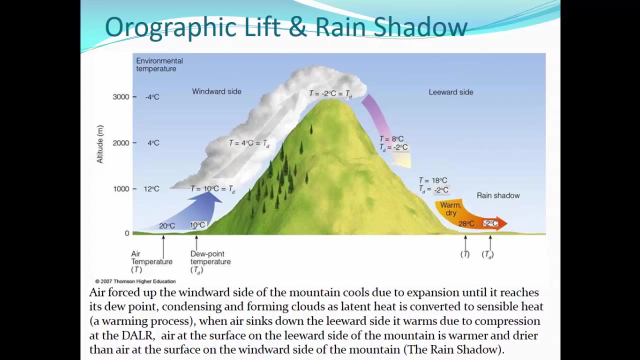 the warm air is moving over a cooler surface. Cold at the surface, warm aloft, that's a stable environment and you get those nice layered stratus clouds. So on this slide we're going to tie all of this together. We're going to have some orographic lift. 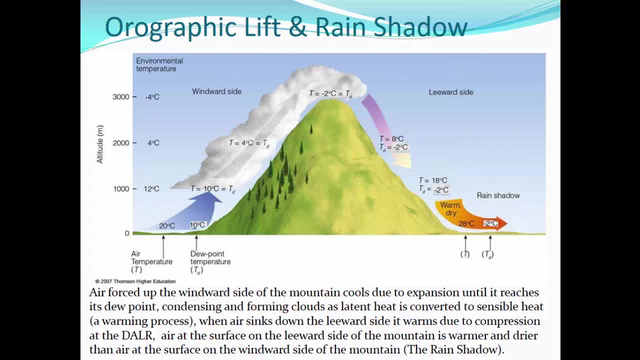 That orographic lift is going to produce clouds, perhaps some showers and what is known as the rain shadow effect And this is going to tie in the adiabatic lapse rate and wet adiabatic lapse rate cloud formation. the whole nine yards. 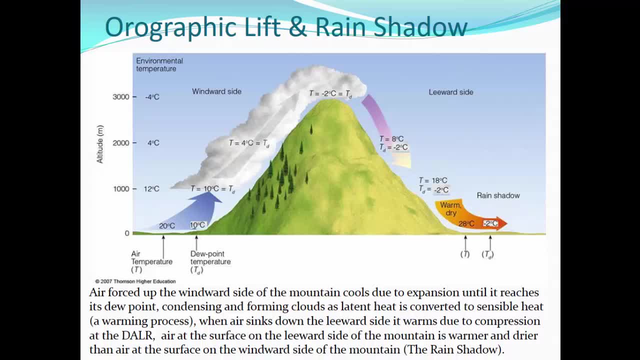 So let's just look at this picture. The wind is blowing from the west, and so it's going to force the air up the west side of that mountain and then force back down the east side of the mountain. So what happens At the surface? 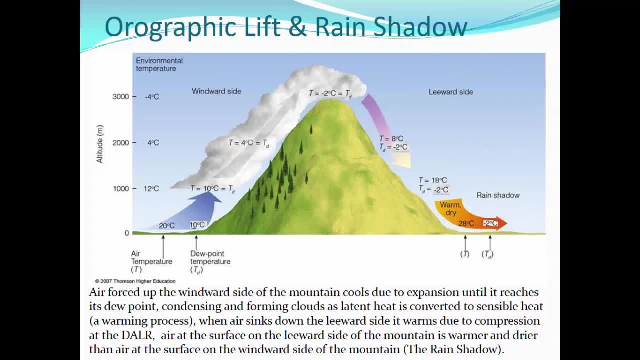 our air has a 20 degree Celsius temperature and a 10 degree Celsius dew point. When we lift that parcel orographically to 1,000 meters, the environment has cooled to 12 degrees Celsius, from 20, 20 to 12 degrees Celsius. 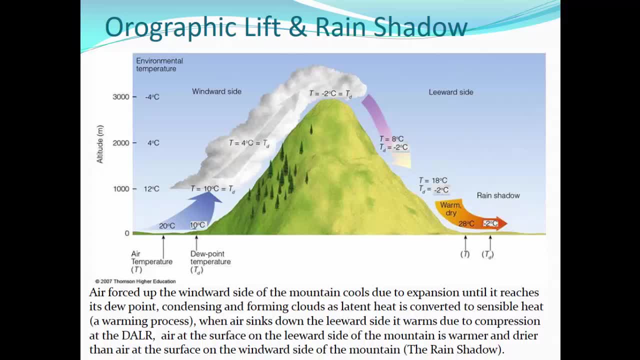 and the parcel has cooled to 10 degrees Celsius. In addition to the parcel cooling to 10 degrees Celsius, it has now also reached its dew point. So the first 1,000 meters of parcel cool to the dry adiabatic lapse rate to 10 degrees Celsius. 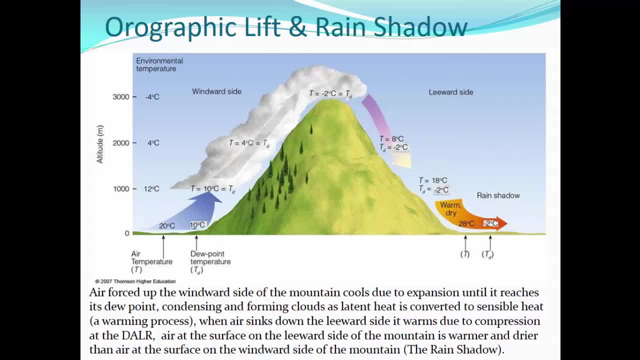 it's now reached its dew point. Further lift up the mountain is going to mean 100% relative humidity saturation and condensation and clot formation. So here goes the lift from 1,000 to 2,000.. The environmental lapse rate. 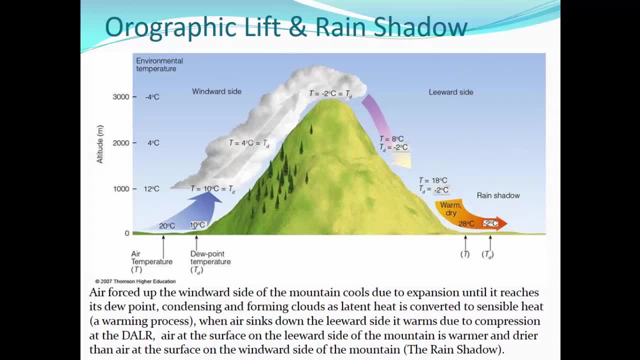 the temperature drops to 4 degrees Celsius and the moist adiabatic lapse rate, the parcel drops to 4 degrees Celsius. But I want you to notice something: Not only does the temperature of the parcel drop to 4 degrees Celsius. 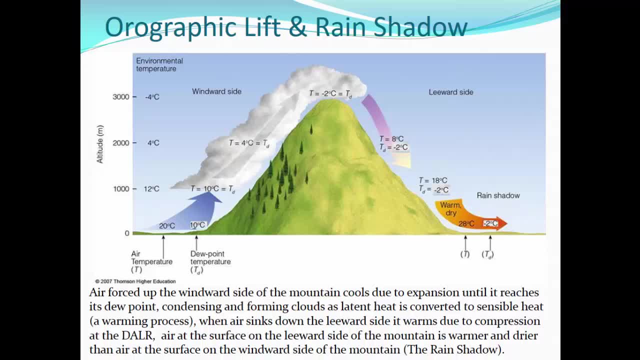 but the temperature of the dew point also drops to 4 degrees Celsius. So what you have to imagine is the dew point is at 10 degrees Celsius at the surface. That is an absolute measure of the amount of water vapor in the air. But when that water vapor, starting at 1,000 meters, 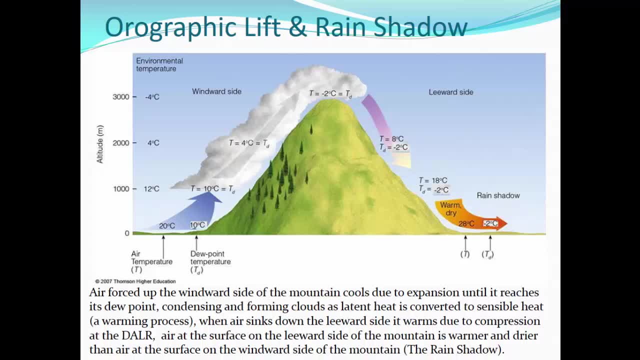 condenses into water droplets, it's no longer water vapor from the air. So, while you may be changing it- a change of state from vapor to liquid, from vapor to a cloud vapor that you can't see, to water droplets that form a cloud that you can see- 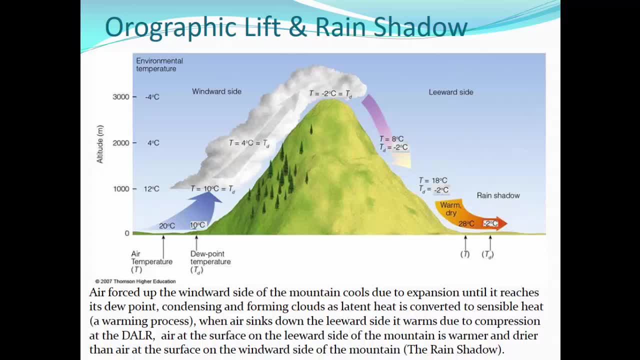 it's still there, but it's no longer in the vaporous form, So the water vapor has decreased. So as the temperature drops from 10 degrees Celsius to 4 degrees Celsius, the dew point also drops to 4 degrees Celsius- another 1,000 meters of lift. 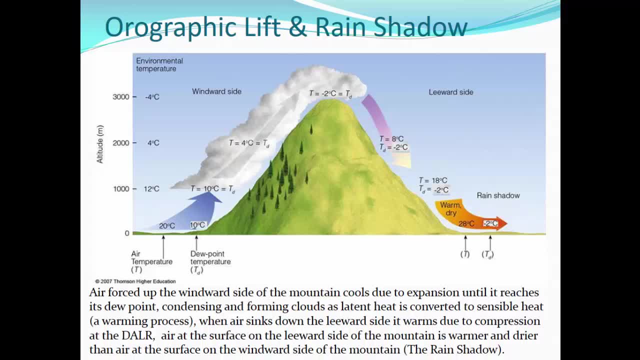 and our temperature drops from 4 degrees Celsius to minus 2 degrees Celsius, and the environmental lapse rates drop now to 4 degrees Celsius, So that parcel is warmer and continues to rise up the mountain. and you can see that not only is the temperature, 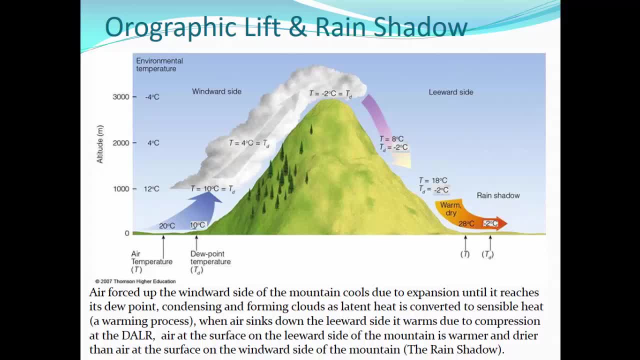 gone from 4 degrees to minus 2,, but the dew point has gone from 4 degrees to minus 2.. Now here's the rub: As soon as you begin to push that air down the lee side of that mountain, the moment you begin to push it down. 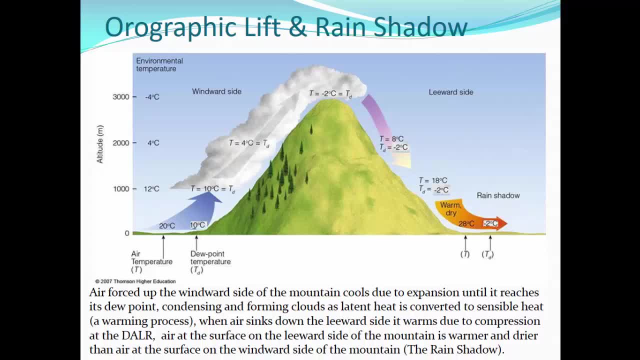 compression warms the air. So if in the first 100 feet, let's say, or 100 meters, the temperature of that parcel warms from minus 2 degrees Celsius to, let's say, minus 1.9 degrees Celsius, 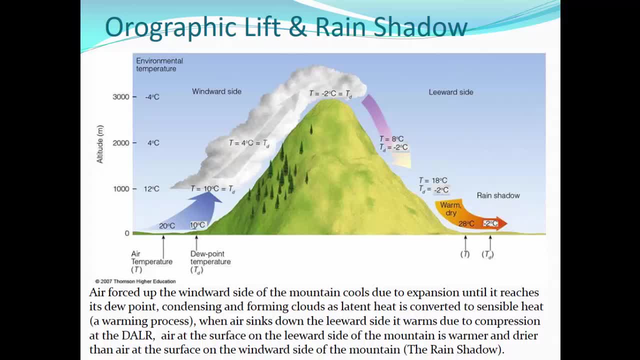 the dew point hasn't changed. More moisture has not been put in that dew point, So that dew point is now lower, lower than the temperature. and so now we are no longer saturated, We are no longer at 100 percent relative humidity. 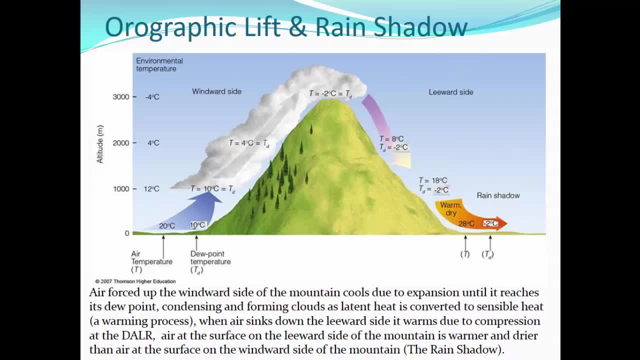 Even if we've only dropped to, let's say, 99.9 percent relative humidity, we now are warming the parcel at the dry adiabatic lapse rate. So look what happens to the temperature as it goes down 1,000 meters. 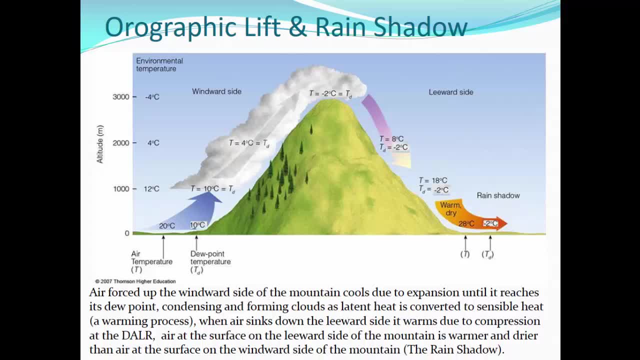 The temperature goes from minus 2 Celsius to 8 degrees Celsius, but the dew point remains the same. No additional moisture is put in the air. Another 1,000 meters down, the temperature goes to 18 degrees Celsius. The dew point stays at minus 2 degrees Celsius. 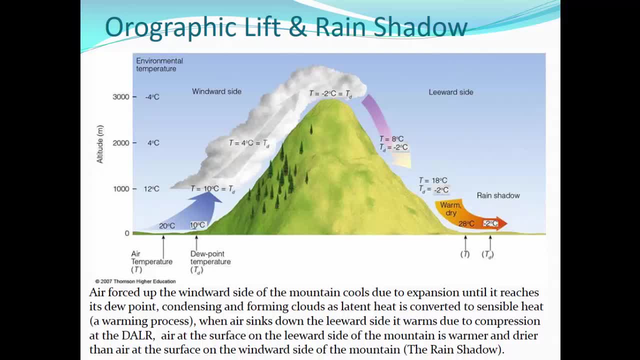 And then another 1,000 meters. the temperature goes to 28 degrees Celsius- actually fairly warm, and the dew point is still at minus 2 degrees Celsius. very, very, very dry, And so you've taken what was fairly mild. 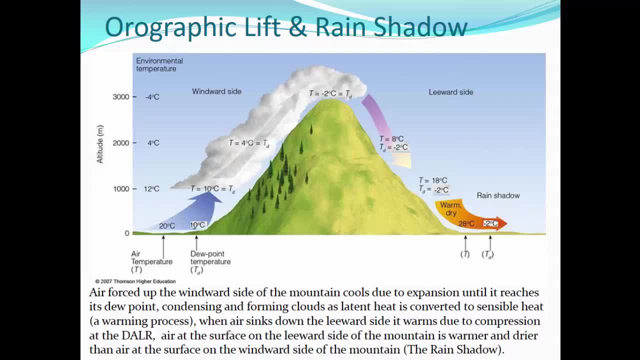 and fairly humid air on the left side, the windward side of the mountain, and you've turned it into very warm and dry air on the leeward side of the mountain, And that's why you don't have the rain on the leeward side. 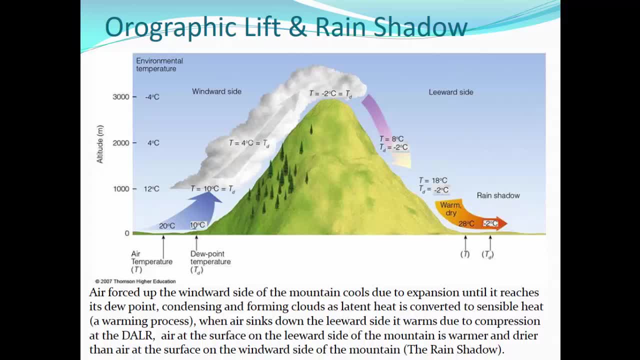 and that's where you get your rain shadow. Air forced up the windward side of the mountain cools due to expansion until it reaches its dew point, condensing and forming clouds As latent heat is converted to sensible heat, a warming process. 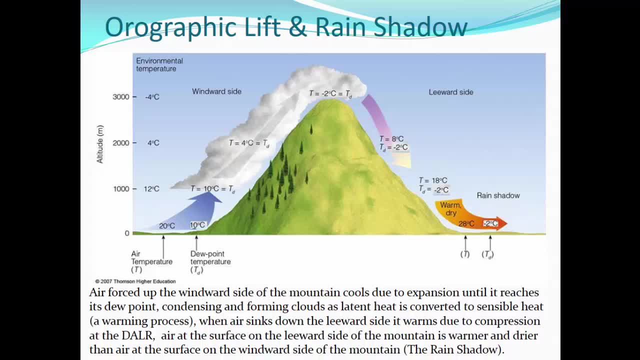 When the air sinks down the lee side of the mountain, it warms due to compression at the dry adiabatic lapse rate. Air at the surface on the leeward side of the mountain is much warmer and much drier than the air at the surface on the windward side of the mountain. 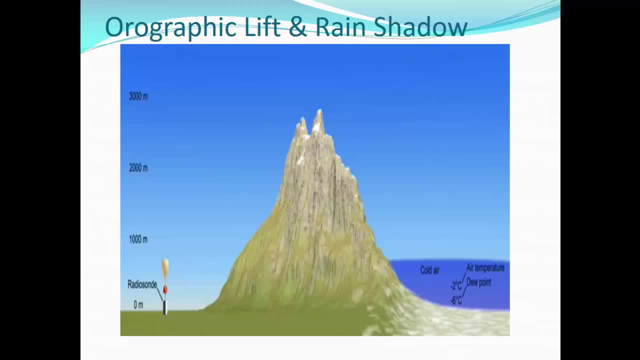 and that is your rain shadow effect. As air rises up along a mountain, it may cool to its dew point, forming a cloud. The release of latent heat inside the cloud warms the rising air. This situation causes the air inside the cloud at the top of the mountain to be warmer. 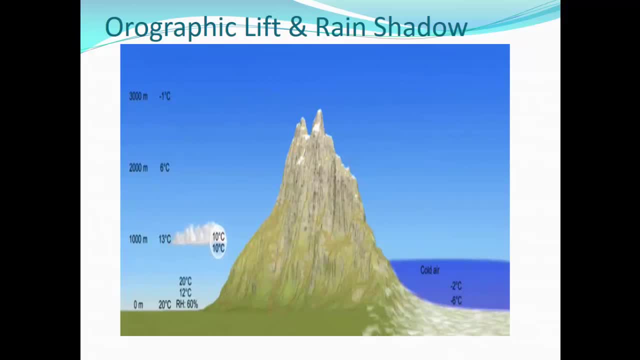 than it would be otherwise. Condensation, and perhaps precipitation on the mountain's upwind side removes moisture from the rising air, so that the rising air at the top of the mountain is also drier. If the rising air at the top of the mountain should descend the mountain's leeward side, 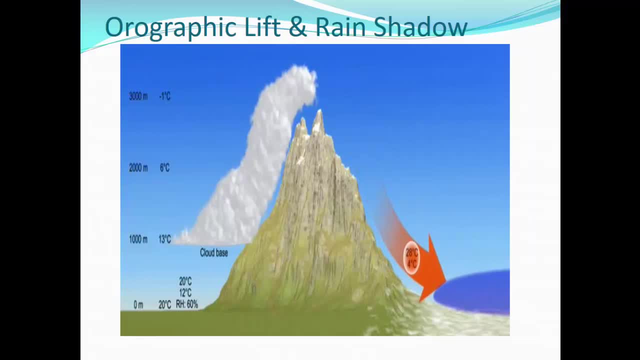 it would produce a warm, dry downslope wind that may replace cold air embedded in low-lying regions. This sinking warming air may also inhibit the formation of clouds and precipitation, producing a rain shadow effect. At this point we should understand. 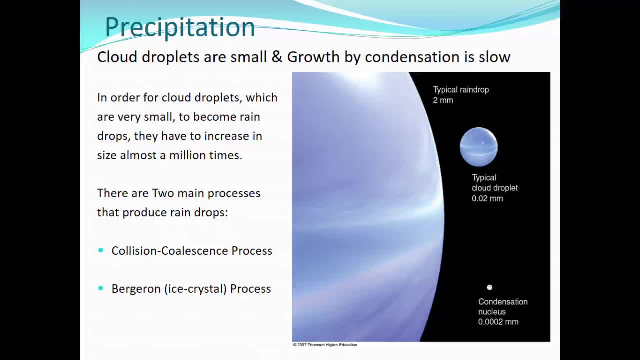 stability and instability in cloud formation, Cloud formation occurring one more time as the air parcel is lifted with a relative humidity of less than 100%, lifted to its dew point at which it reaches 100% relative humidity saturation, further lifting, creating condensation and cloud formation. 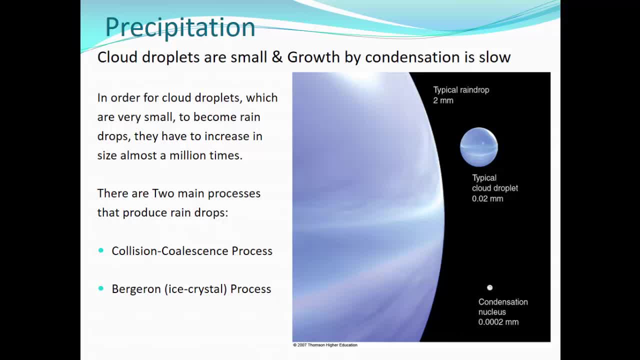 So you have a cloud. So what does that mean? Well, look at this picture. The typical cloud droplet about 0.02 millimeters across, where the typical raindrop is 2 millimeters across, And so we're talking about almost a million times larger. 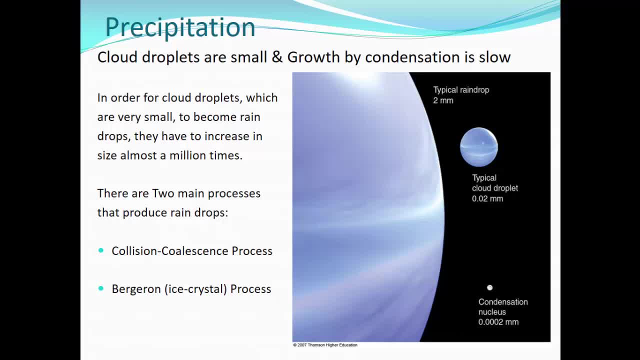 So how do we get from cloud droplets to raindrops? Cloud droplets have to get really big, really fast in order for clouds to produce rain. Well, two main processes: One's known as collision and coalescence and the other is known as the Bergeron process. 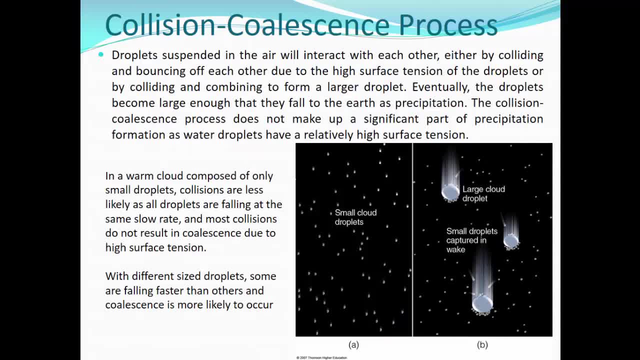 but more typically known as the ice crystal process, Two methods. One is to get cloud droplets into raindrops big enough to fall from the sky. The first one, of course, the collision-coalescence process: Literally droplets colliding together and coalescing. 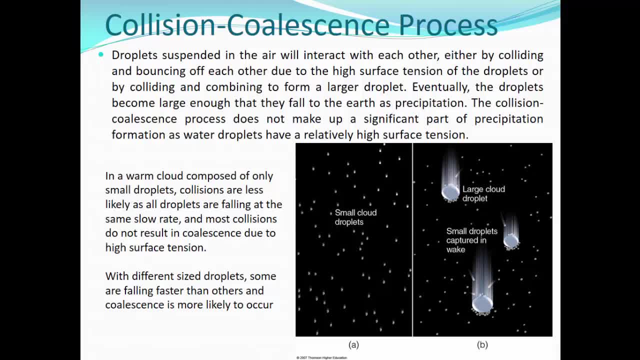 Coalescing, essentially meaning joining together. Droplets suspended in the air will interact with one another, either by colliding and bouncing off of one another- because well tiny little water droplets have a very high surface tension- or by colliding and combining to form larger droplets. 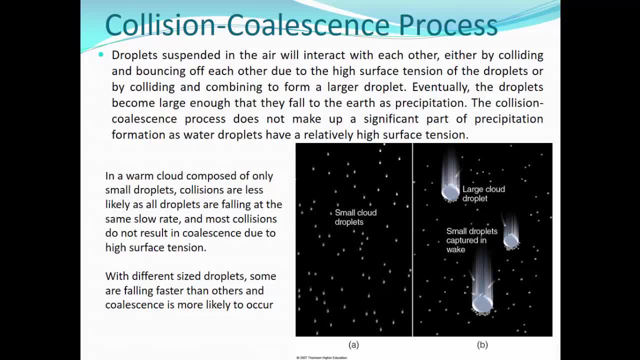 Eventually the droplets will become large enough that they fall to Earth as precipitation. But the collision-coalescence process one is a pretty slow process and it really does not make up a significant part of precipitation formation, because water droplets do have that relatively high surface tension. 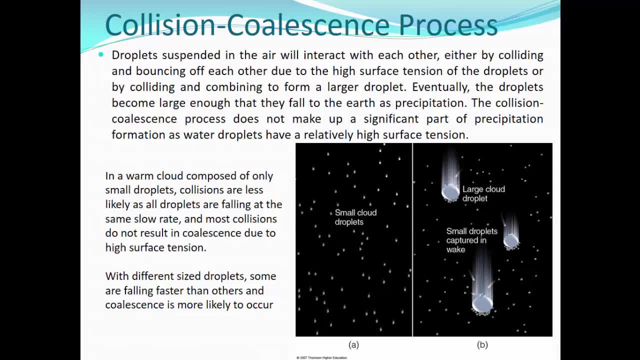 So in a warm cloud composed of only small droplets, collisions are really less likely, as all the droplets are falling and moving at the same slow rate and most collisions do not result in coalescence due to high surface tension. You have to have a larger, deeper, thicker cloud. 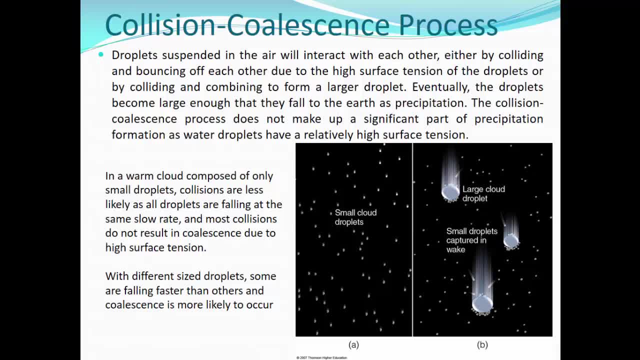 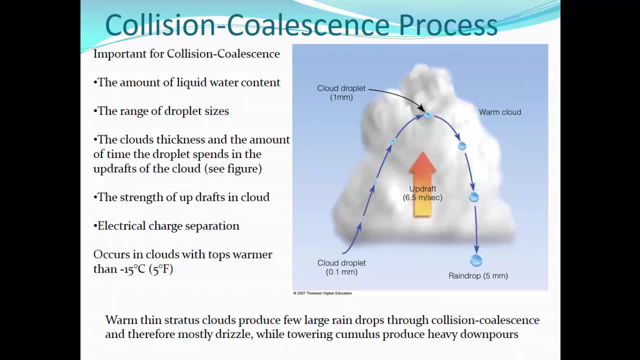 with different sized droplets, where some are falling a little bit faster than others, to actually get coalescence to occur. So there are some important factors that have to be in place in order to get collision and coalescence to occur. A lot of it has to do with the clouds. 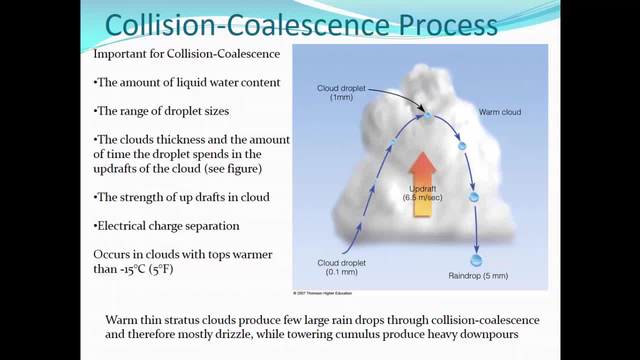 being clouds of vertical extent or cumulus clouds. Cumulus clouds tend to produce the rainfall where low warm stratus clouds. they may hang there all day long and make the day very gray, but they don't generate a lot of precipitation. 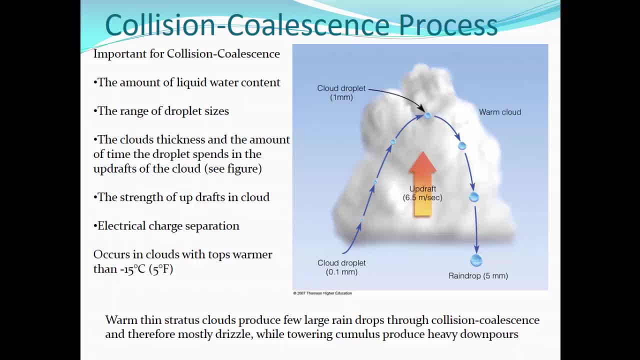 So what's important for collision and coalescence? The amount of liquid water content. You've got to be in an area with lots of humidity, so clouds have lots of liquid water, And there's got to be a range in droplet sizes. 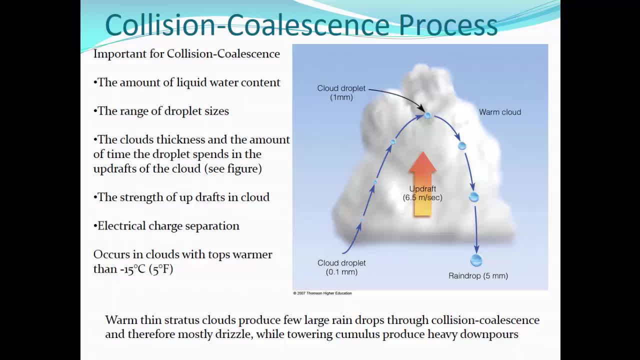 and that again goes back to that upward vertical motion that creates those clouds of vertical extent. Clouds have to be thick and the amount of time the droplet spends in the updraft has to be large. So with an updraft that droplet has to get pushed up for a long time. 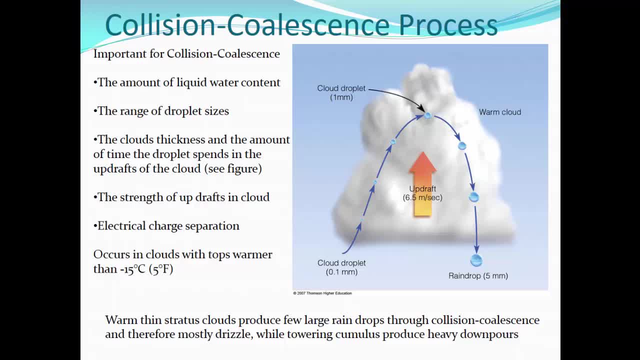 and be able to fall for a long time in order to grow large enough to fall as precipitation. So that requires a strong updraft within the cloud. It helps if there's an electrical charge separation, which we'll talk about later on this semester when we get into lightning. 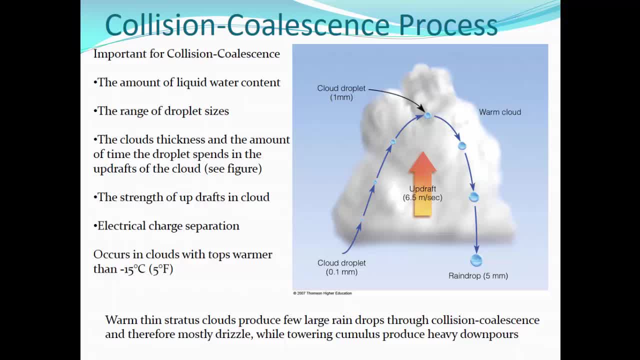 And typically this occurs in clouds with tops that are warmer than 15 degrees below zero Celsius and 5 degrees Fahrenheit, which you can tell is below freezing. But again, and we've talked about this before, water droplets can occur in the atmosphere sub-freezing. 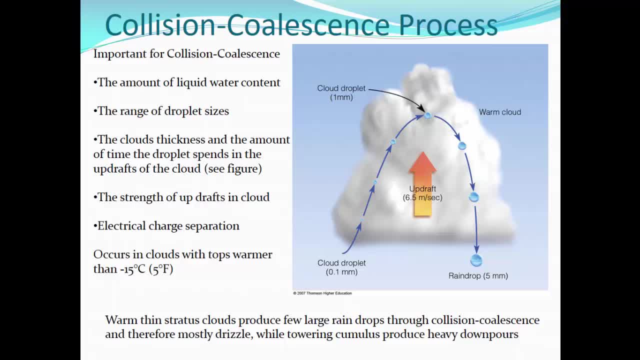 If they don't have condensation nuclei or they don't have freezing nuclei to freeze to water droplets in the atmosphere can chill below freezing. As a matter of fact, they can get to as much as 40 below freezing before they will spontaneously freeze. 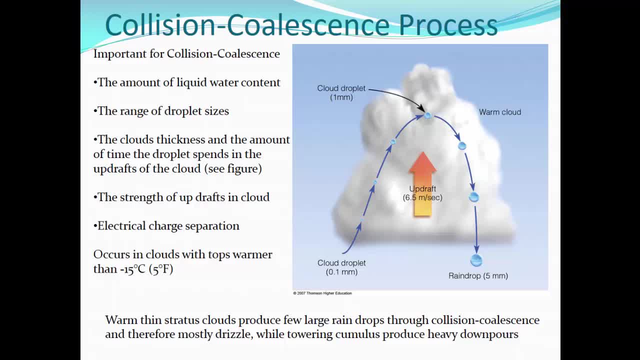 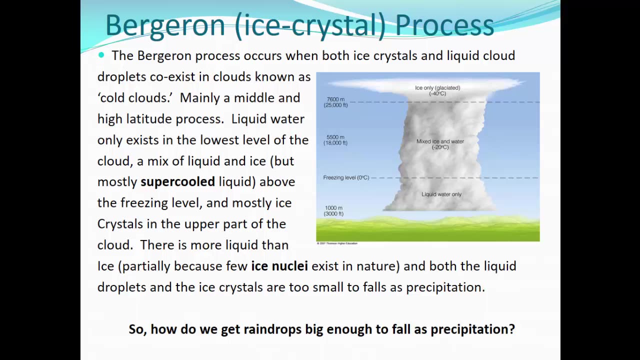 So warm, thin stratus clouds produce very few large raindrops through collision and coalescence and therefore only really that drizzle And towering cumulus. with strong updrafts they can produce those very heavy downpours, So the ice crystal process occurs. 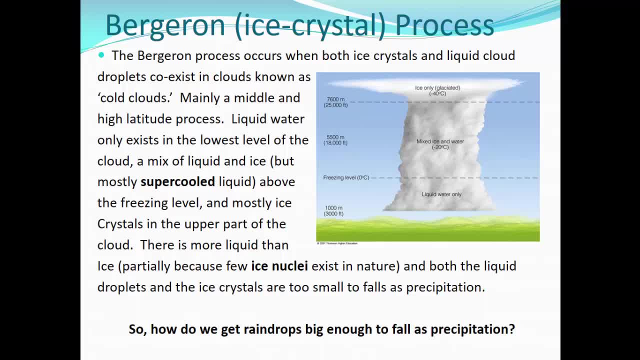 when there are both ice crystals and liquid cloud droplets coexisting in clouds known as cold clouds, mainly in the middle and higher latitudes, And we find that mixed ice and water layer somewhere above the freezing level in the middle levels of the atmosphere. 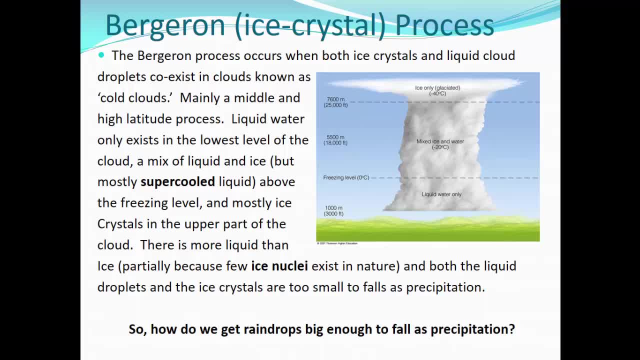 Now you get way up above the atmosphere, 25,000 feet or higher- and you start to get to a point where there's only ice in the clouds. up there, Clouds are called glaciated, but we're looking at this much larger area. 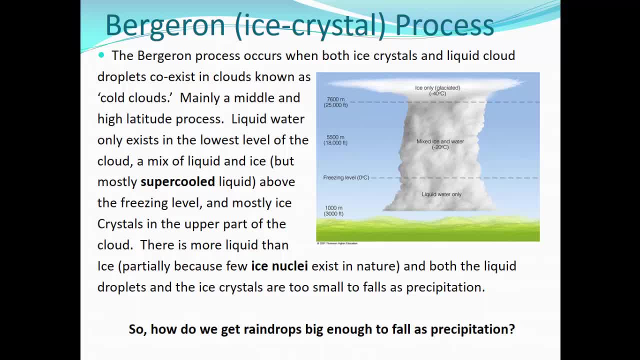 in our towering cumulus clouds between the freezing level and 25,000 feet, that mixed ice and water level. Liquid water only exists in the lowest levels of the cloud, where it's only liquid water, The mix of liquid and ice, but mostly supercooled liquid. 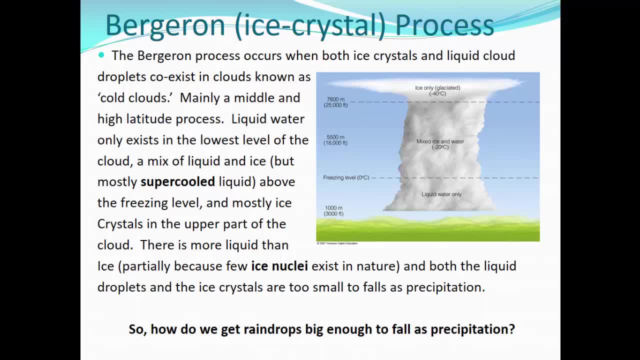 again liquid below freezing, above the freezing level, and then mostly ice crystals. in the upper part of the cloud There is more liquid than ice, partially because there's just not a whole lot of ice nuclei in nature. So in that mixed ice and water layer 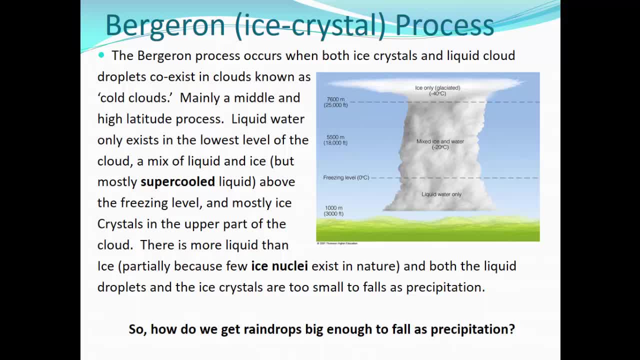 there's a lot of liquid and a little bit of ice, and both the liquid droplets and the ice crystals are too small to fall as precipitation. So how do we get raindrops big enough to fall as precipitation? That's the ice crystal process. 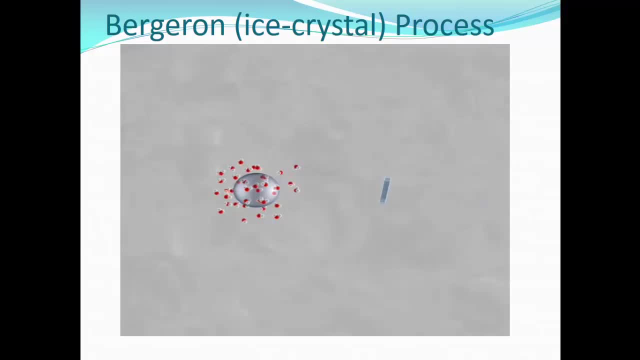 Inside a cloud where temperatures are below freezing, ice crystals may be surrounded by supercooled water droplets. When ice crystals and liquid droplets are close together, water vapor molecules will move from the liquid droplets and deposit onto the ice crystals. 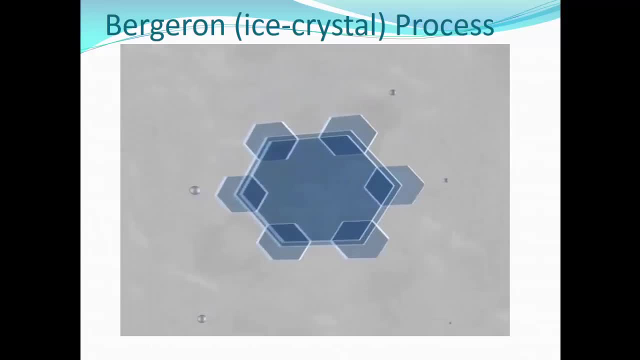 This situation causes ice crystals to grow in size while water droplets shrink. When an ice crystal becomes significantly large, it begins to fall. While falling, the ice crystal may grow in size by colliding and sticking to other ice crystals or by colliding with supercooled droplets. 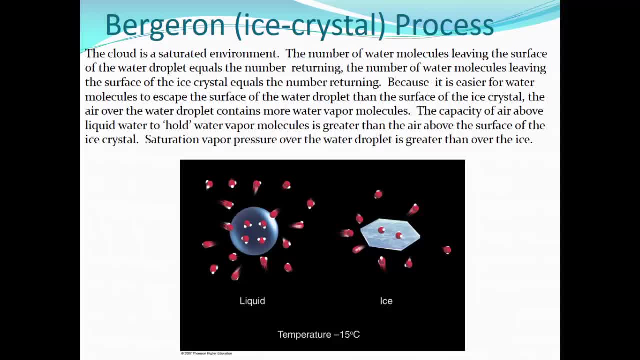 The details of that ice crystal process. the cloud is a saturated environment. If it's a cloud, the relative humidity is 100% and we have a condensation and cloud formation going on. The number of water molecules leaving the surface of water droplets. 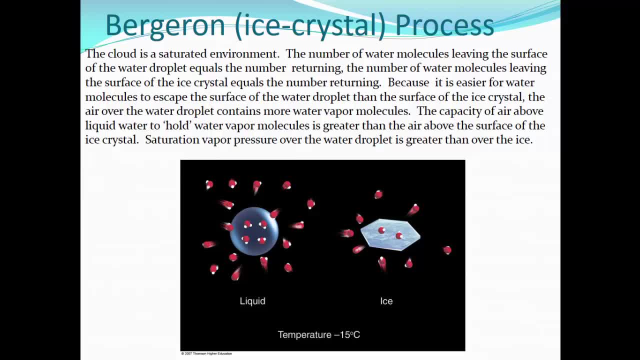 is equal to the number returning, and the number of water molecules leaving the surface of ice crystals is equal to the number returning. Remember- that is the definition of saturation: that there is a certain amount of water and a certain amount of saturation, That there is the same number of molecules. 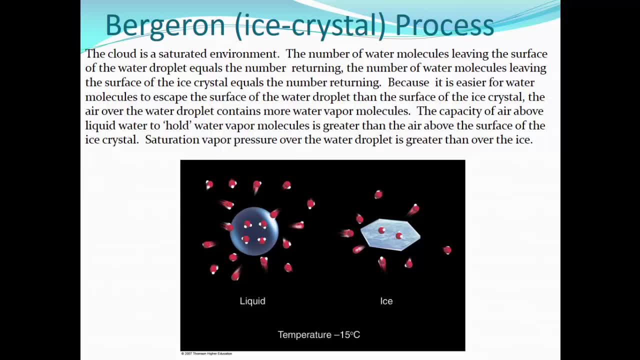 leaving the liquid water as exiting the liquid water surface and the same number of molecules leaving the ice as growing to the ice. That's the definition of saturation, But because it's easier for water molecules to escape the surface of the water droplet. 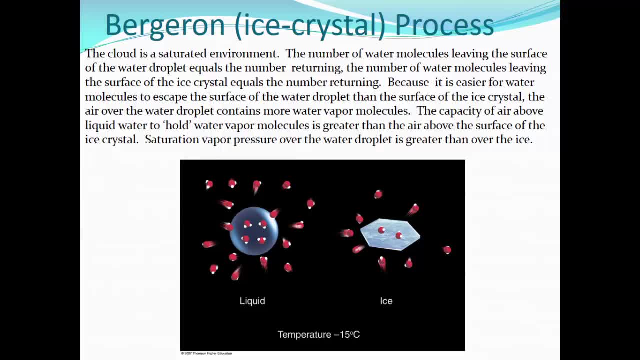 than the surface of the ice crystal. the air over the water droplet contains more water vapor molecules. If you remember our chart, it was a while back- on saturation- vapor pressure- saturation vapor pressure over the liquid water was higher than over the ice. 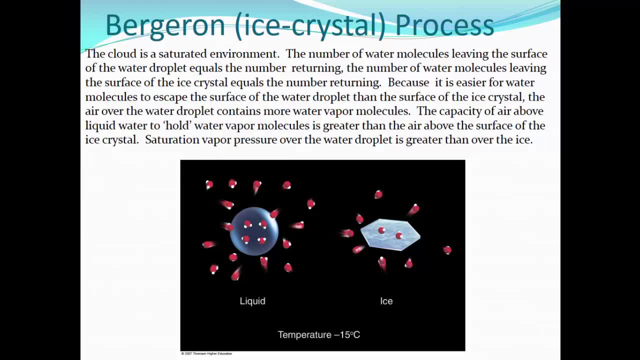 There are more molecules around that liquid water than around the ice, And so there's a gradient. There's a gradient with higher numbers of molecules in the air over the liquid and lower numbers of molecules in the air over the ice. And because of that gradient, 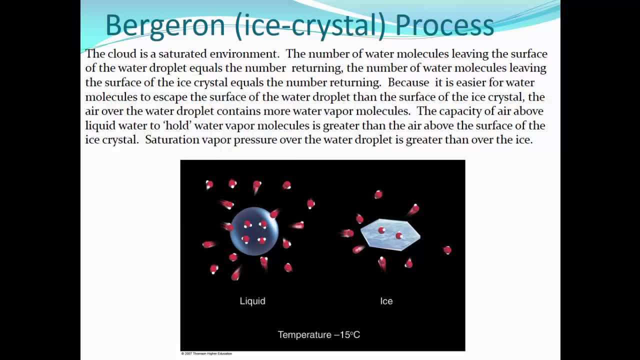 the molecules travel from the liquid to the ice. So, because it's easier for water molecules to escape the surface of the water droplet than the surface of the ice crystal, the air over the water droplet contains more water vapor molecules. The capacity of the air to hold water vapor molecules 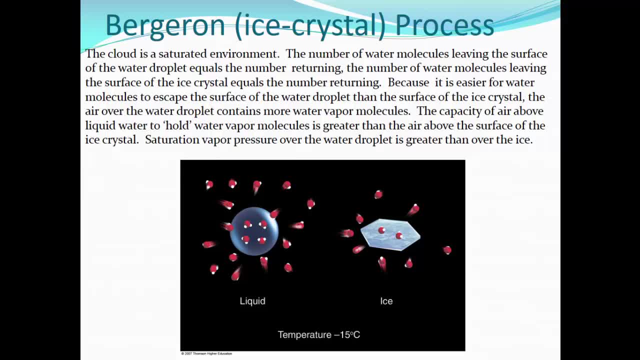 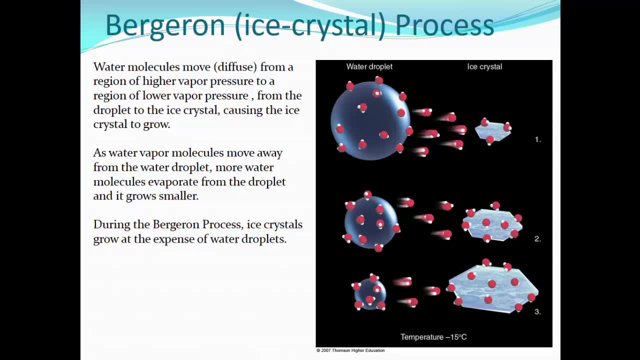 is greater than the air above the surface of the ice crystal. Saturation: vapor pressure over the water droplet is greater than over the ice crystal. Again, whenever there is a gradient, mass will want to move from higher to lower If it's a gradient of a hill. 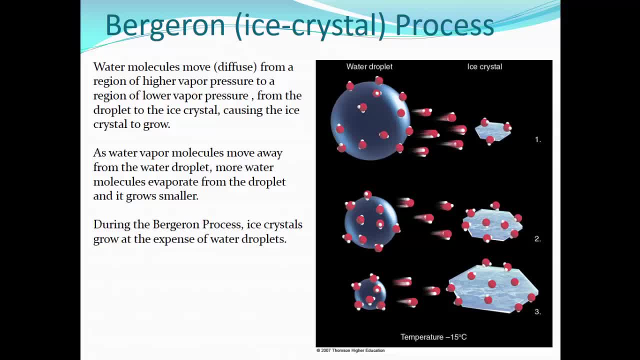 the skateboard at the top of the hill will go from the high to the low elevation If it's pressure at the surface. wind will blow from higher to lower, From high pressure to low pressure If it's a gradient between high saturation, vapor pressure over water. 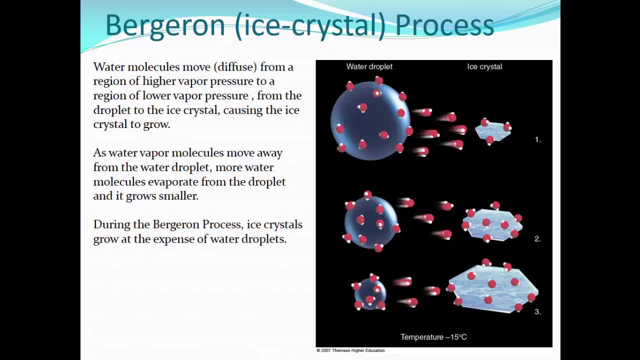 and lower saturation vapor pressure over ice, then water molecules will move from the region of higher vapor pressure to the region of lower vapor pressure, from the droplet to the ice crystal, causing the ice crystal to grow As water vapor molecules move away from the water droplet. 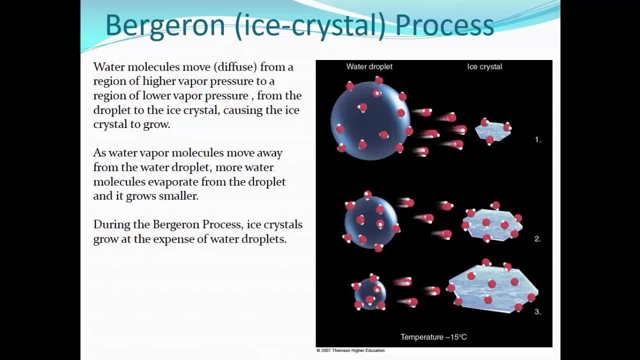 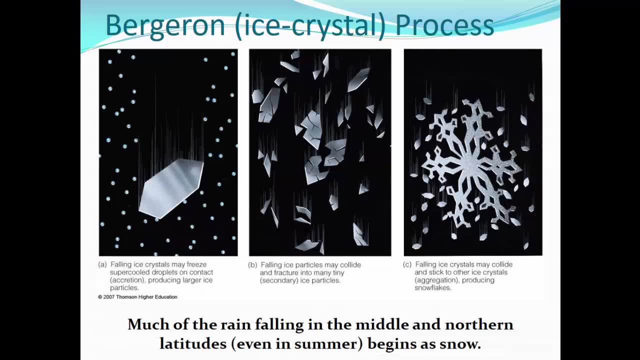 more water molecules can evaporate from the droplet and the droplet gets smaller. During this process, ice crystals grow at the expense of water droplets. Because of the ice crystal process, much of the rain falling in the middle and northern latitudes 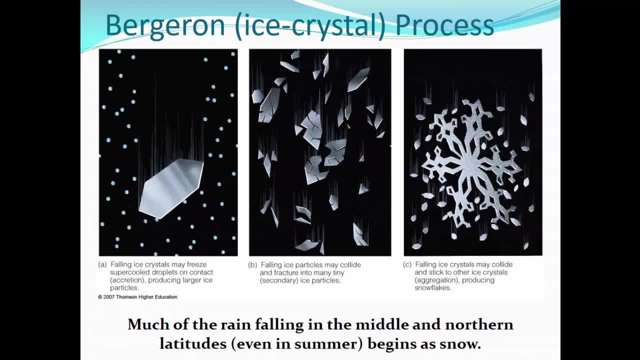 even in the summertime, begins as snow. So again, falling ice crystals may freeze supercooled droplets on contact, producing larger ice crystals. Those crystals can bang into each other and fracture and break apart, and then all those little itty-bitty pieces of crystals. 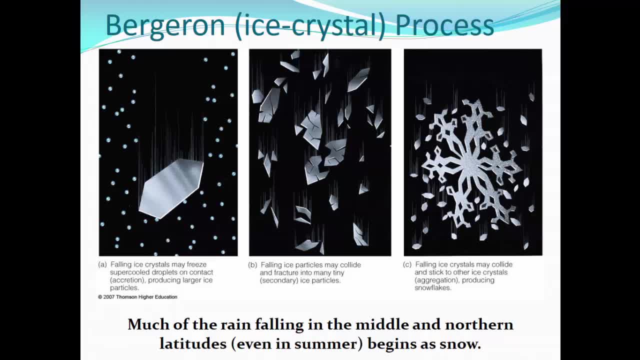 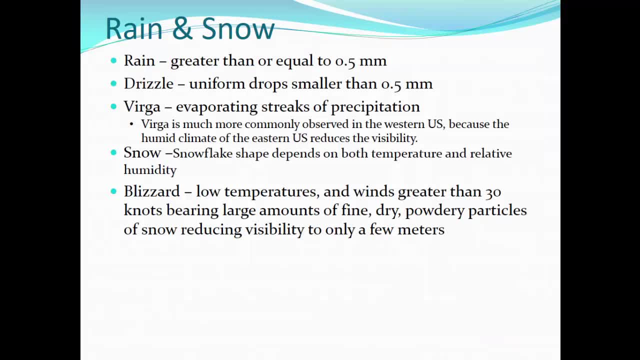 can stick back together to produce bigger snowflakes. So again, this process is going on in the cloud, but essentially most of our rain begins as snow or ice. Different types of precipitation: rain, drizzle, virga, snow and blizzards. 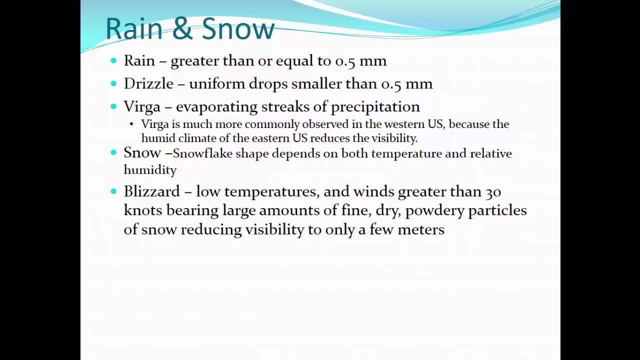 Rain is, of course, droplets that are greater than or equal to half a millimeter. Drizzle, then uniform drops that are smaller than half a millimeter. Virga is actually rain falling from the base of the cloud that evaporates before striking the ground. 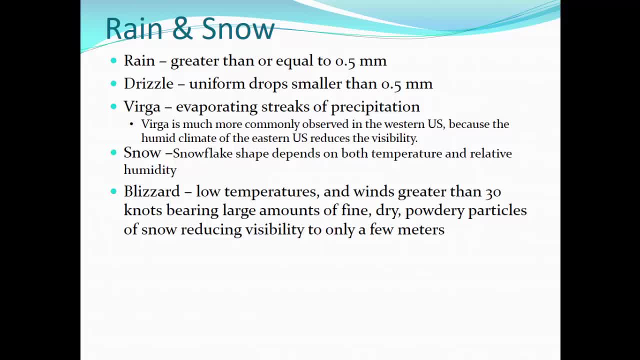 Typically that happens in your drier climates. but you can see the fall streaks. You can see the rain coming out of the cloud and then evaporating. Of course, evaporation is a cooling process. Cool air is heavier, So under those types of storms out west, 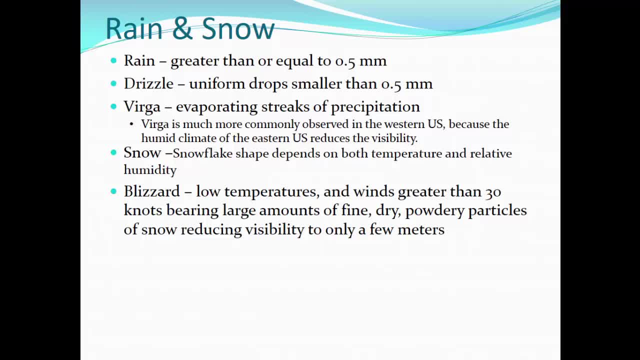 you get a rush of cold air and sometimes you get what's referred to as dry microbursts. Very, very cold air rushes, the ground spreads out, creating some damaging winds, but there's no rain. that comes with it Snow and, of course, snowflake shape. 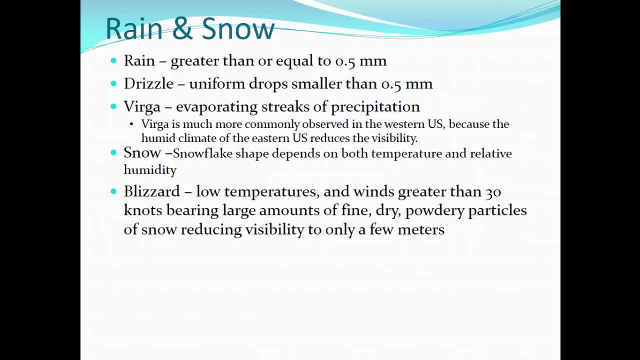 depends on both temperature and relative humidity and blizzards. And blizzards have little to do with the amount of snow but much more to do with how much wind is blowing, because the high winds will blow all that fine powdery snow. 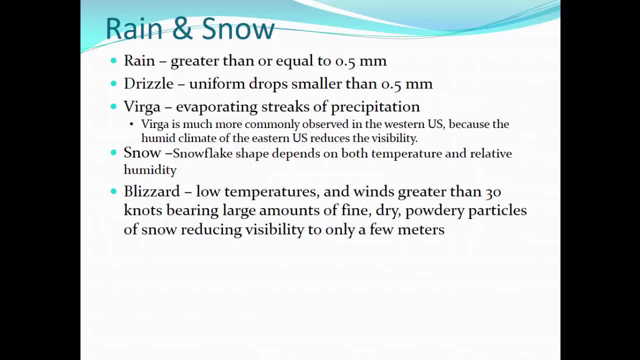 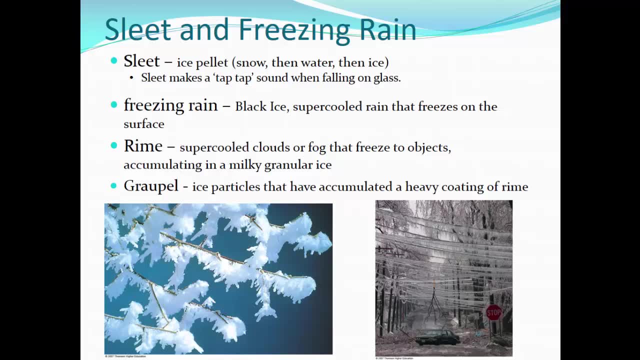 to reduce the visibility to only a few meters. So blizzard's more about the wind blowing snow to reduce the visibility to only a few meters? Your types of frozen precipitation sleet, which are actually little ice pellets, That is snow that melted to water. 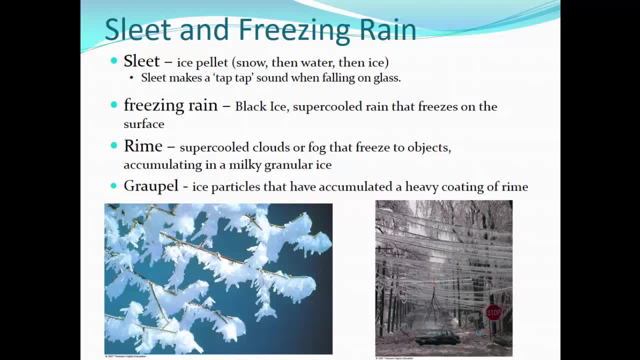 and then refroze. Sleet tends to make this tap-tap sound when falling on glass like your windshield. Freezing rain- not sleet at all, but freezing rain- is also called black ice. That is super cold rain, so raindrops that may be at or below freezing. 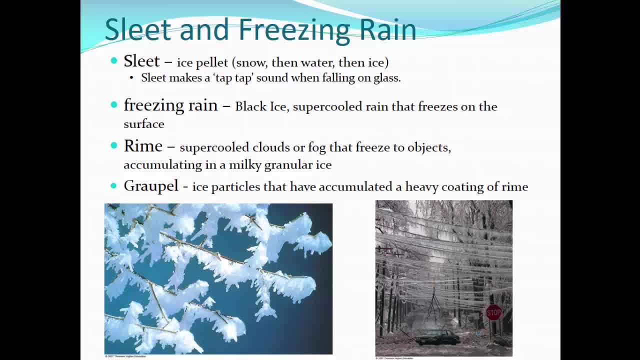 that fall as liquid but then freeze instantaneously when they strike objects in the ground. That's where we get ice storms from. Rime is a little bit different. That's on the left. Rime is super cool: clouds or fog that freeze the objects. 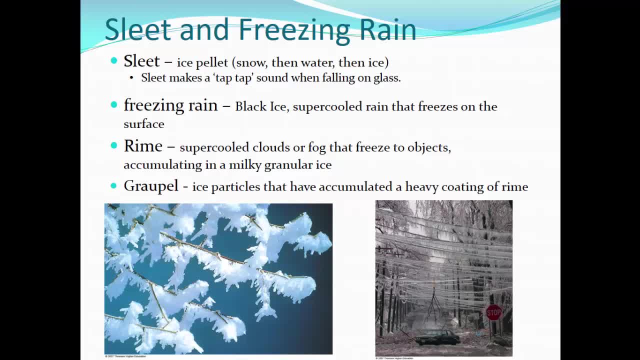 and that's where you get like icing on airplanes. It's a super cold fog or clouds, so tiny droplets It's not actually falling as precipitation and it just accumulates on an object and creates this milky, granular ice. 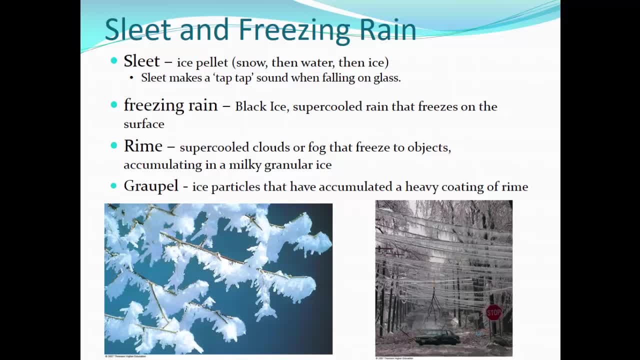 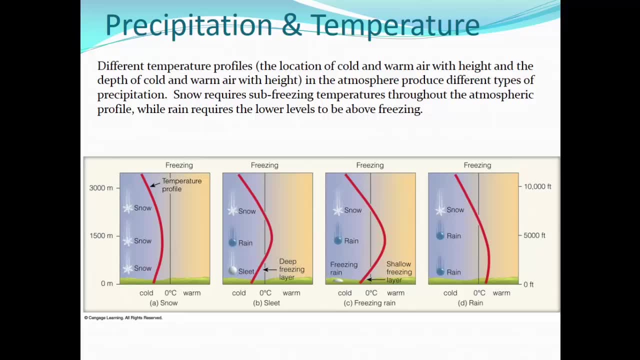 And then graupel are ice particles that have accumulated a heavy coating of rime, which is just kind of a subtle difference in frozen precipitation. But those different types of frozen precipitation require different temperature profiles. The state of the atmosphere has to be different. 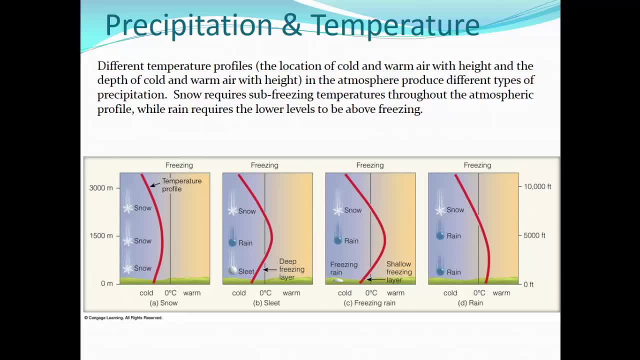 to get different types of frozen precipitation. Different temperature profiles, the location of the cold and warm air with height and the depth of that cold and warm air with height produce different types of precipitation. Snow requires sub-freezing temperatures throughout the atmospheric profile. 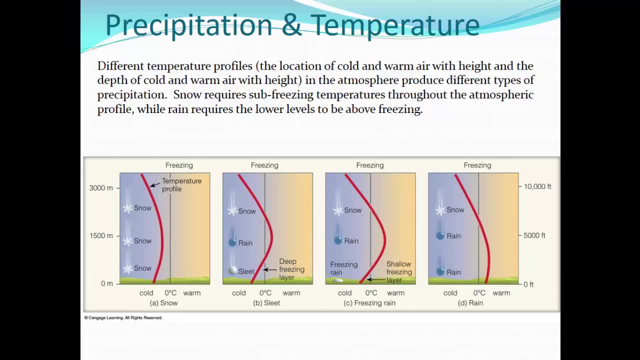 while rain requires the lower levels to be above freezing. So look at the illustration on the far left, The entire column of the atmosphere is below freezing. It starts as ice falls, as ice hits the ground, as ice. where on the right, 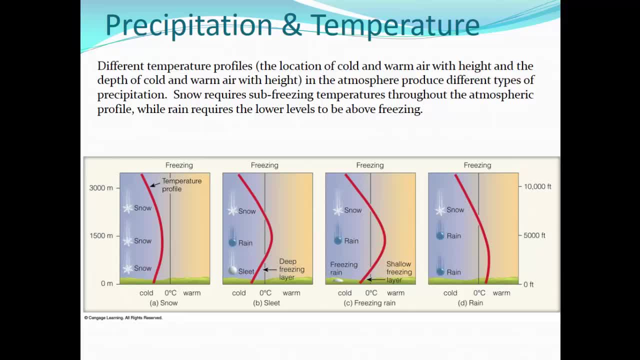 the upper levels of the atmosphere are below freezing and then you get a thick, very deep warm layer where that snow melts to rain, And then in between you get sleet and freezing. sleet and freezing rain And the biggest difference between sleet and freezing rain 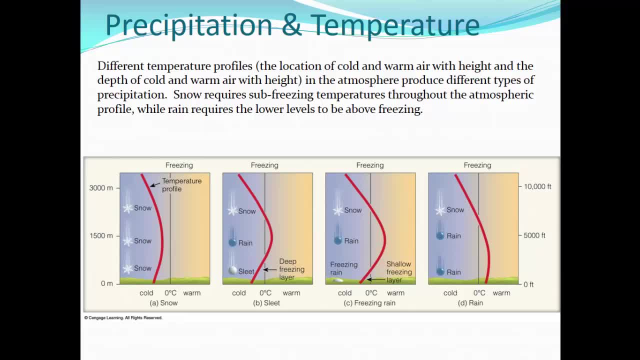 is that with sleet you have this deep freezing layer at the surface. The middle layers of the atmosphere are warm enough that the snow melts to rain, but then you have a deep freezing layer where that raindrop refreezes into a pellet. 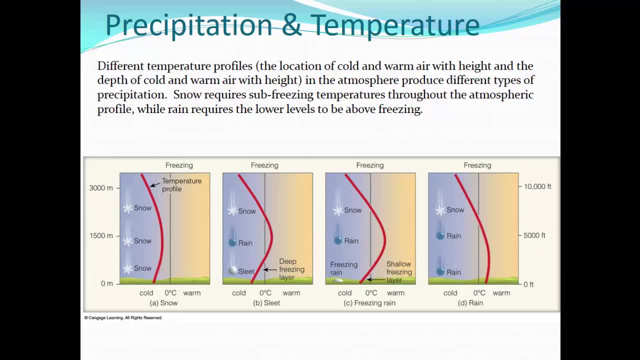 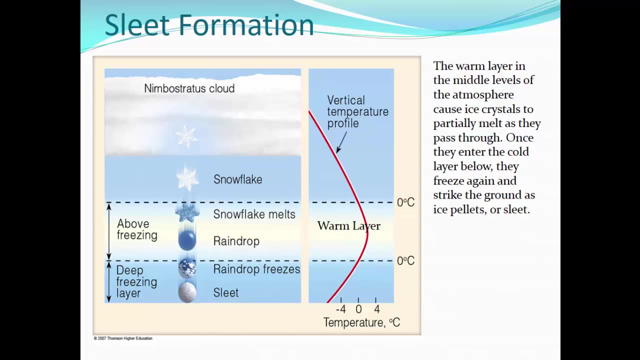 Whereas with freezing rain, that black ice snow turns to rain because of a mid-level warm layer, and then a very, very shallow freezing layer causes that rain to freeze on contact and that's where you get your very dangerous freezing rain. So again in sleet formation. 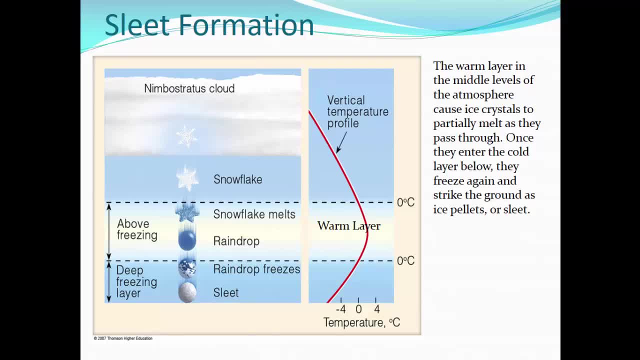 there's your profile of the atmosphere on the right, with below freezing in the low levels, above freezing in the middle levels and then below freezing in the upper levels, So that warm layer in the middle levels of the atmosphere causes ice crystals to partially melt. 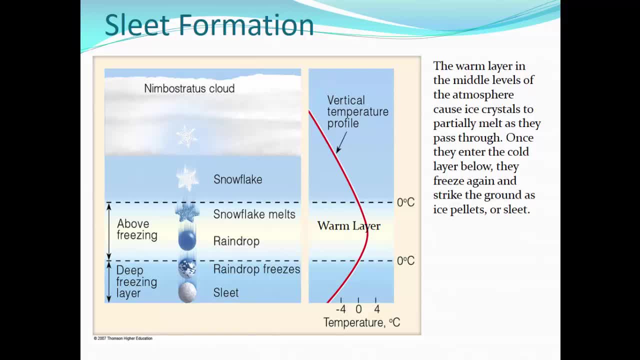 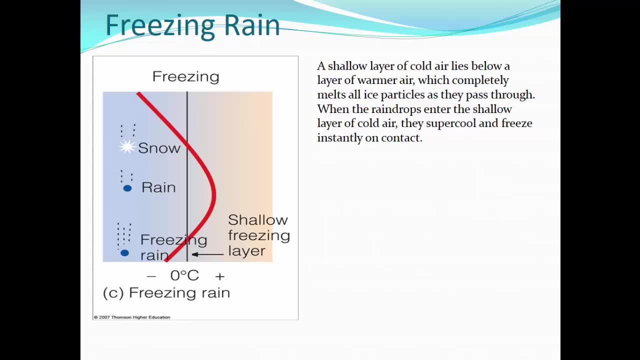 as they pass through. Once they enter the very cold layer below, they freeze again and strike the ground as ice pellets or as sleet Freezing rain- now very dangerous because the rain falls and strikes asphalt and freezes and you don't see it. 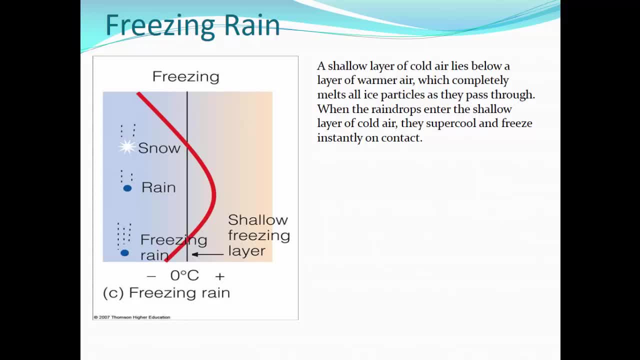 It's clear, It's ice, And so that's where we get this description of black ice And you have frozen roads, very, very dangerous. But a shallow layer of cold air lies below a layer of warmer air. That layer of warmer air completely melts. 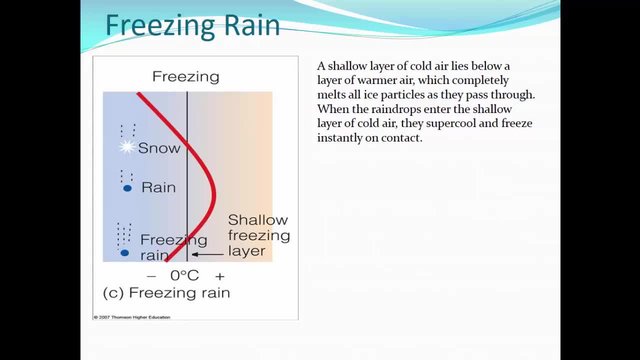 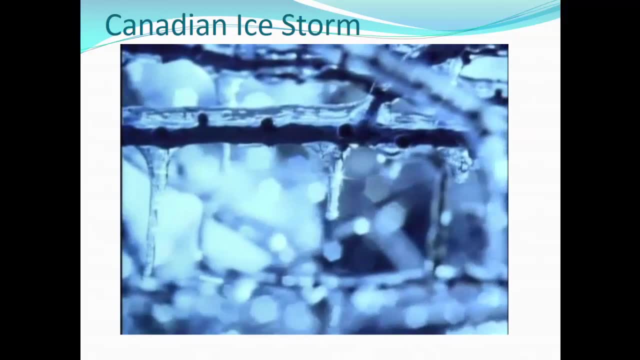 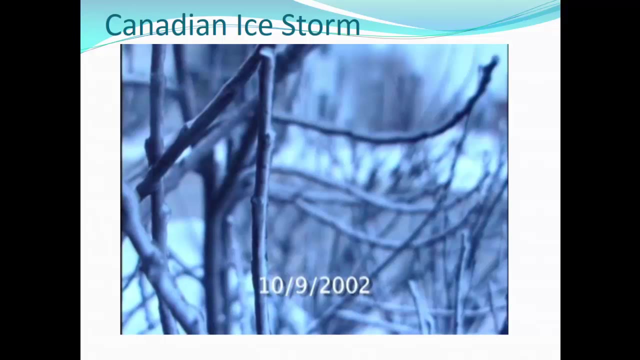 the ice particles as they pass through. So when the raindrop enters that shallow layer of cold air, they super cool and freeze instantly on contact. Ice storms are not unusual in Canada, coating the landscape with a beautiful shroud of ice, But in January 1998,. 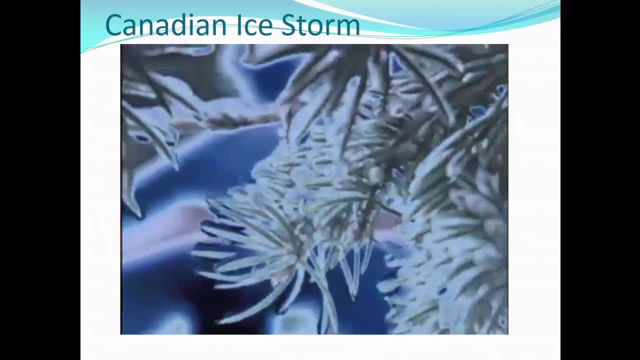 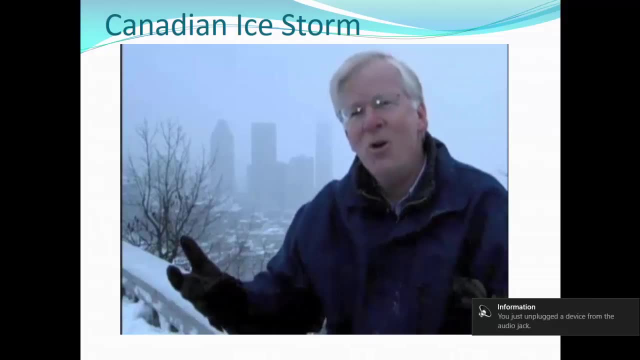 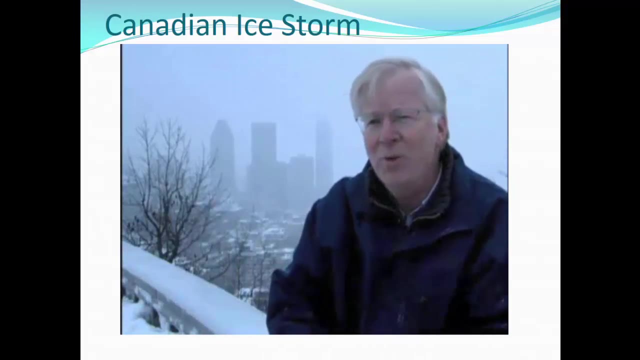 Canada was hit by a storm that was anything but usual At first. the ice storm of 1998 was just as magical. It was really more of an exhilaration. People were not too disrupted by that. School was canceled. You had businesses closed. 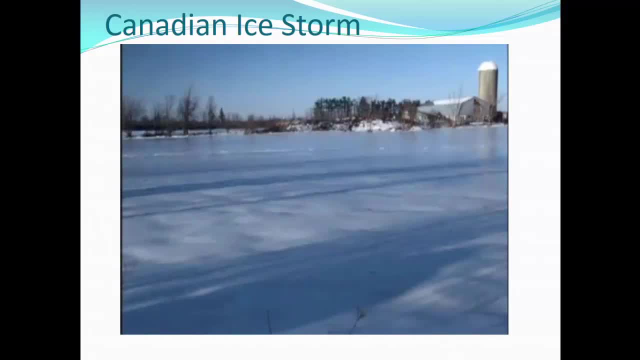 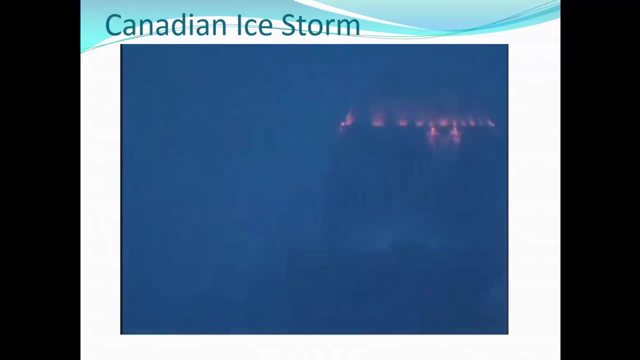 But it was a winter wonderland. It gives you that enchanted wonderland. The landscape looks so beautiful. On the evening of the 4th of January, winter was still on the attack. A bank of freezing polar air sat like a blanket over the northeast of the country. 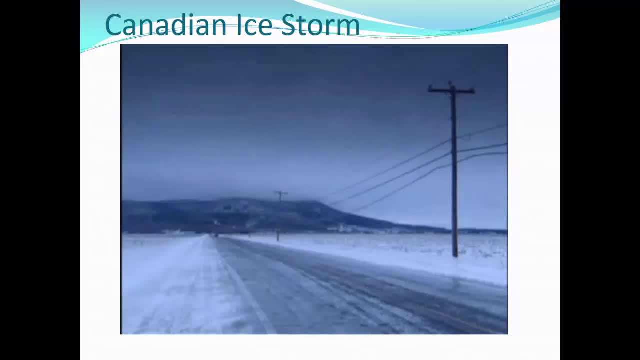 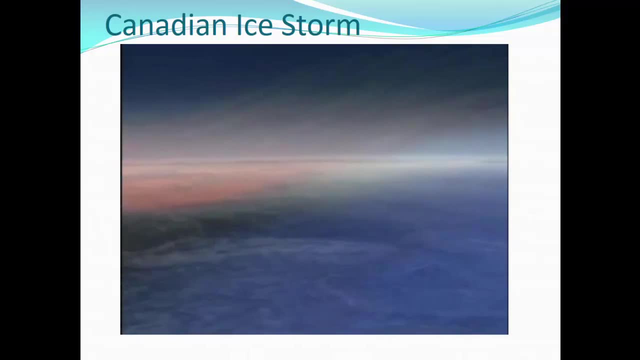 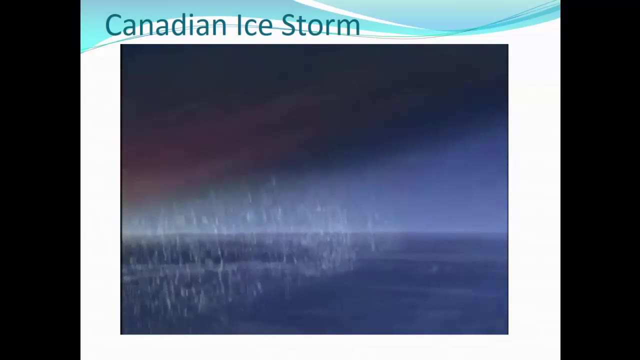 At the same time, a mass of warm, moist air from Texas moved in above the polar air, forming a wedge and trapping it beneath Perfect conditions for an ice storm. But in the middle of the wedge, rain from the warm air above doesn't have enough time to freeze solid on its way down. 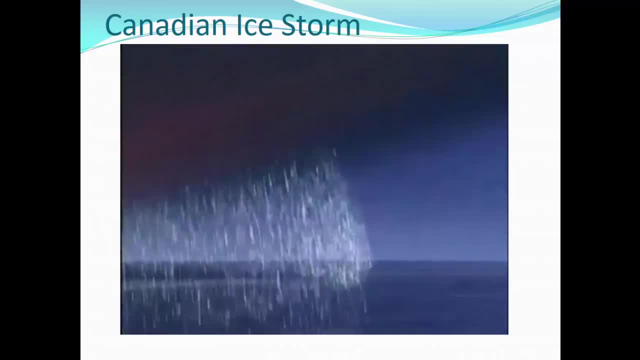 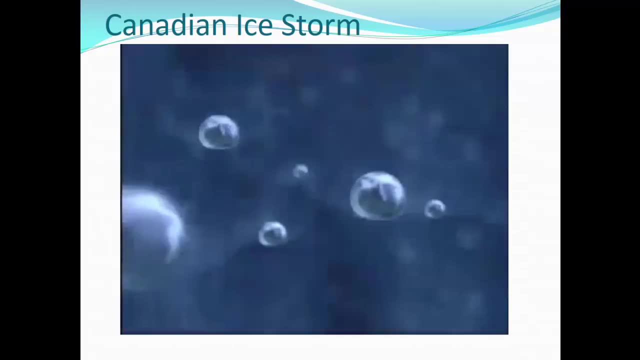 So it folds as super-cooled rain. What happens is that the raindrop will fall through that wedge of cold air and the liquid raindrop that will begin to cool, but it doesn't get quite frozen. It freezes to the point that it's what we call super-cooled. 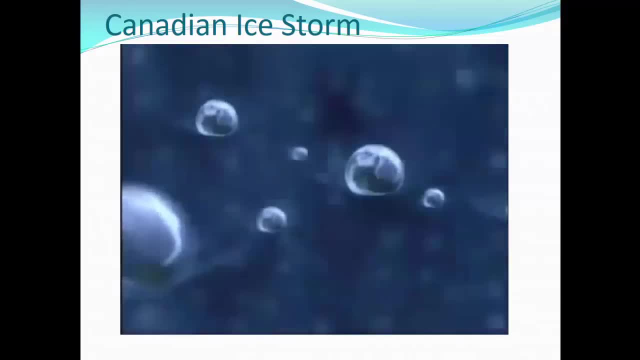 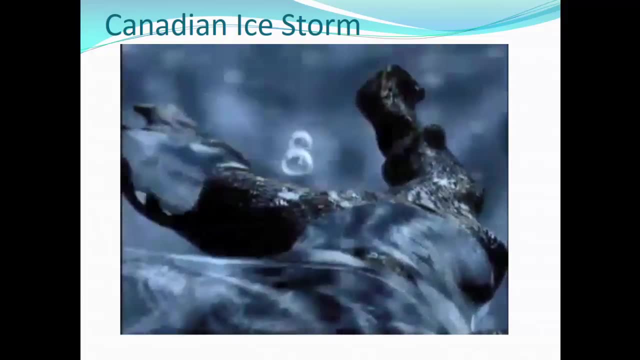 It actually is below freezing. It falls below the freezing point but it's still liquid. And because the object that it hits is below freezing, it's almost shocked. It makes that perfect transformation from the liquid to the solid. It spreads out and freezes into a little veneer of ice. 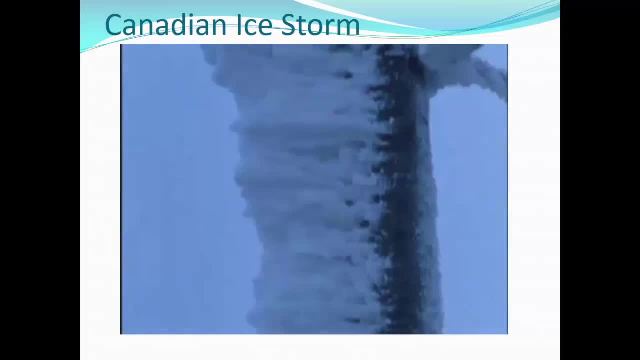 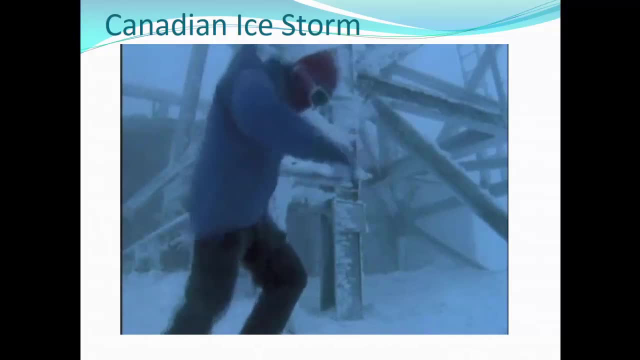 which is the toughest and most adhesive ice that nature can produce. And this ice just kept building up and getting thicker and thicker and thicker and the wires kept going up, And the wires kept getting bigger and bigger, and all of the trees around, of course. 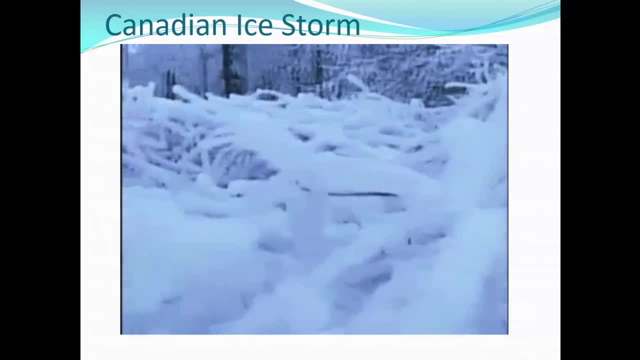 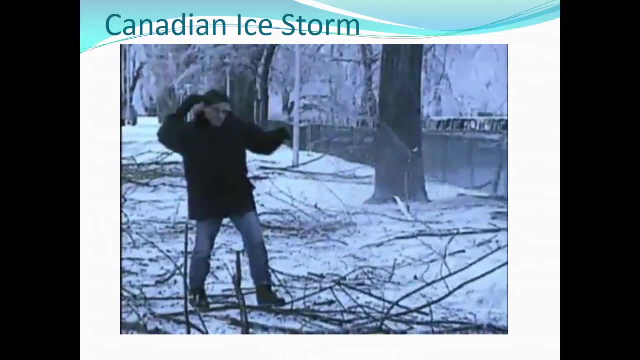 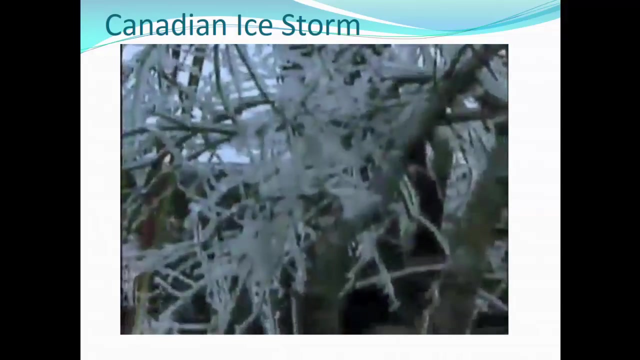 were building up with ice, You could have maybe four inches of ice around a small twig- And of course that twig is part of a branch which is also encased in ice- will all of a sudden have a totally different weight and it will finally break and fall to the ground. 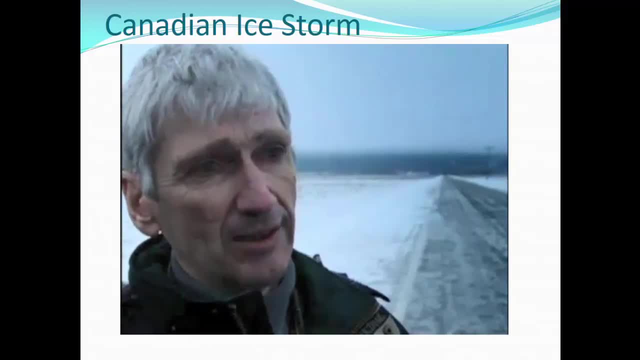 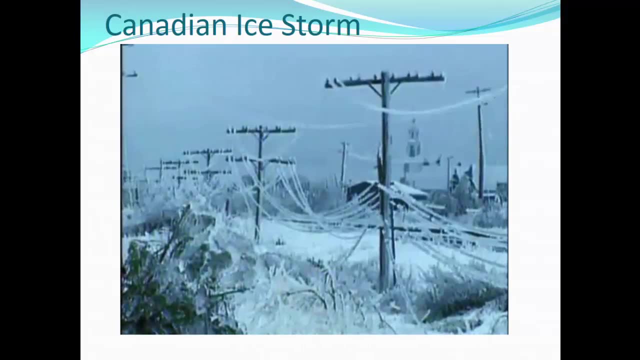 This condition kept up for hour after hour and then, gradually, that's when we started to hear the trees coming down and then the lines started coming down. Trees were falling on the lines, and the lines were falling down on their own because of the weight of the ice. 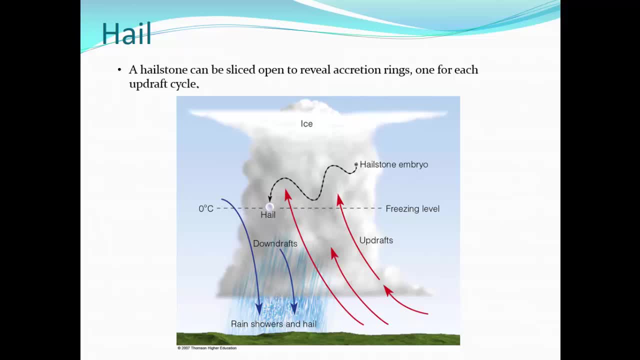 that was building up on there. Now, hail is an entirely different creature altogether. Hail is the case where you have a hailstone embryo. You can see it there in the upper levels of the atmosphere. It's just going to be an ice crystal. 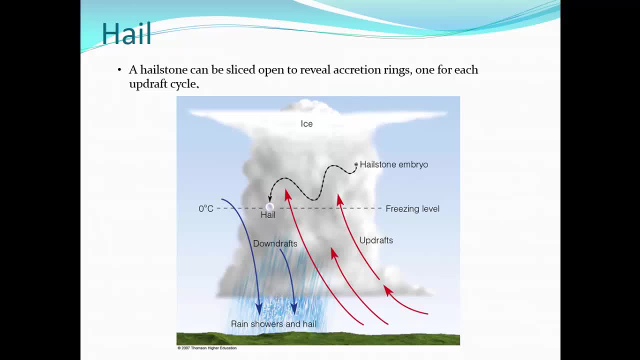 It falls and then it gets into an updraft and it goes back up and then another layer, another layer freezes on the hailstone, so it gets a little bit bigger and it falls again and then another updraft pushes it back up. 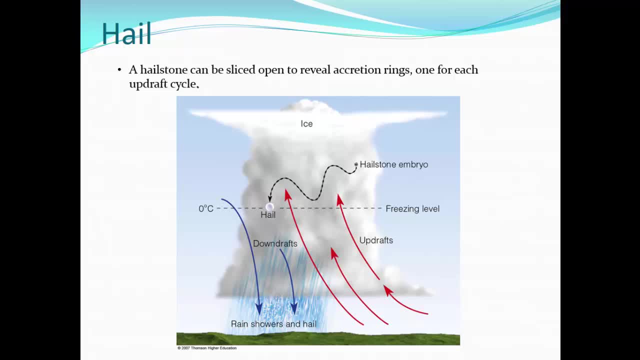 and a whole other layer of ice grows in the hailstone. so it falls again and eventually it gets big enough that it can fall through the updraft, or it gets caught up in a downdraft and falls. But the bottom line is this: hail. 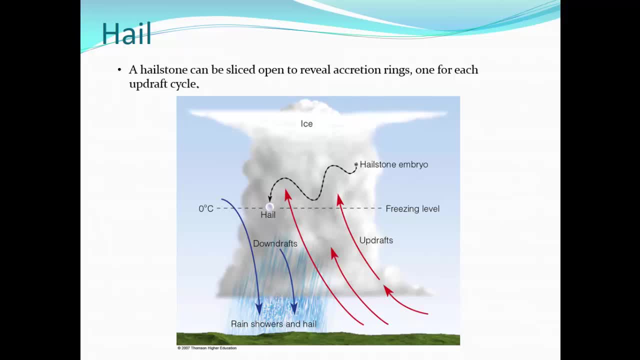 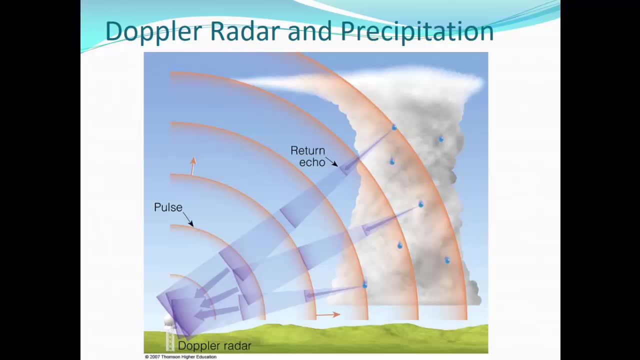 has one layer after the other and the bigger the hailstone. if you can cut it in half while it's frozen, you can actually see the different layers of ice as the hailstone traveled up and down in that thunderstorm. updraft, All right. 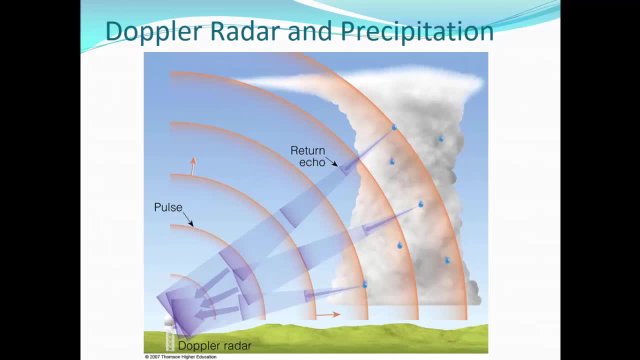 For the end of this lecture. we're going to shift from our stability, our cloud formation and our precipitation and talk a little bit about how we detect our precipitation, which is going to be our Doppler radar, And so on the left.